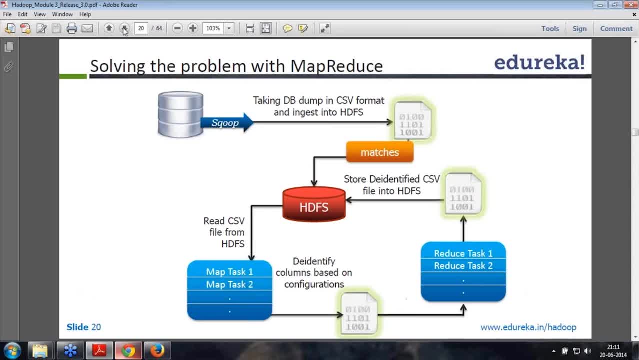 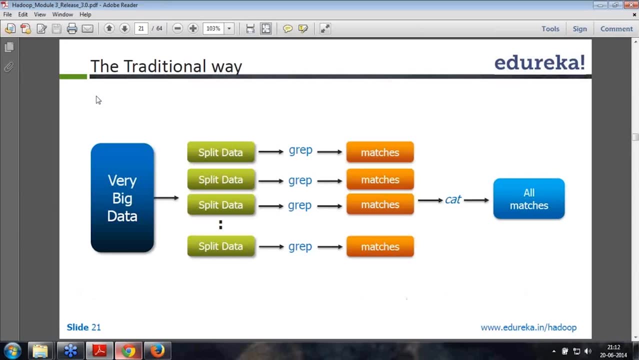 So when you write a code, it will consist of a map and a reduce. Of course, we will have a look at the flow of it also, So, don't worry, I'll explain everything for you folks. So this is how you would solve that particular problem. So now, if you're trying to use a traditional way, not the MapReduce way, you're not using Hadoop, So you have got a huge amount of data. 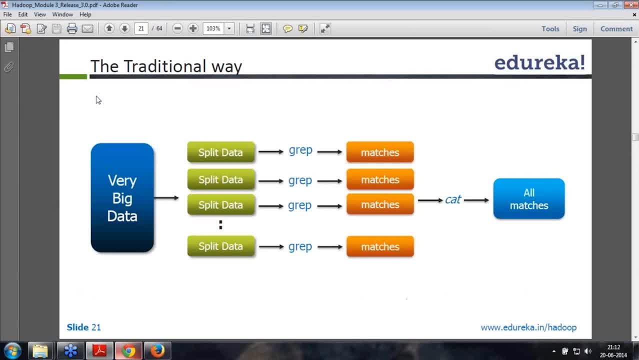 You know that the crux of this thing is parallel processing. If the centralized processing has its own limitations, where everything is happening at one location, So you would need to process it parallelly. So that's the reason why you would have the data split into multiple small chunks. 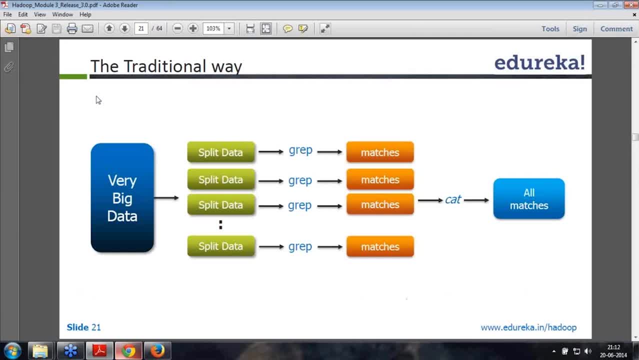 So as a developer you will have to do the splitting, whereas in your Hadoop world the framework does the splitting into 64 MB block automatically. We don't have to write a code for that. but then if you were writing this in the old way, 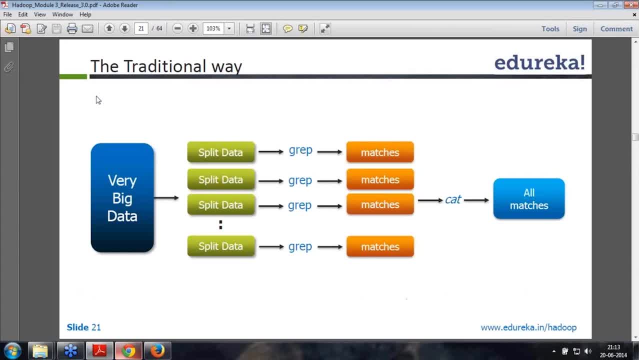 without MapReduce. you have to do the split, Then you have to do a grep and then you have to match. that grep is looking through the data and then matching whatever is the logic that you want to write. You have to ensure that the code is there on each place wherever you have split the. 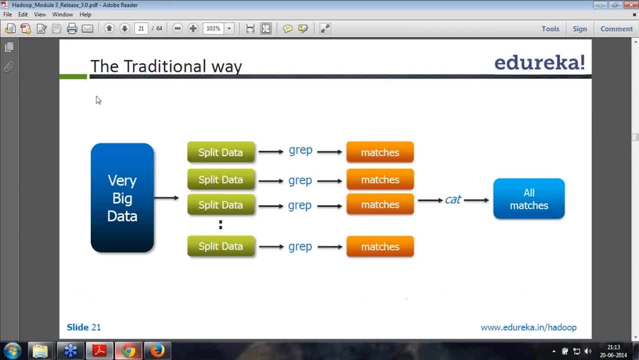 data. Here again, the MapReduce framework does all of these things magically, So the code automatically goes down to the node wherever the data is. After that you have to bring together in the old environment in the traditional way, all the matches together. 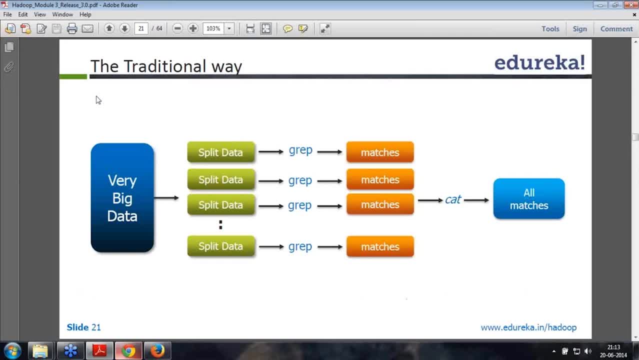 You have to bring it together into one place and then you'll have to accumulate it And again. this is the third thing what the framework does: It brings the data from all the different places where it was done individually and give it to you in a consolidated format in HDFS. 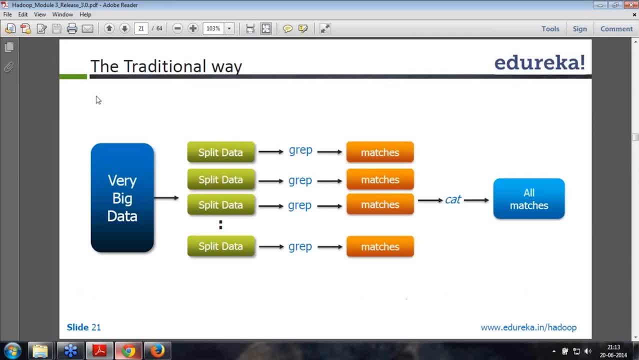 So what does the framework give to you? The ability to split the data automatically, the ability to run the code on the block split wherever the data is splitted. That is what is called as moving code today: Moving code to data, aggregating the data from the multiple places and giving you it. 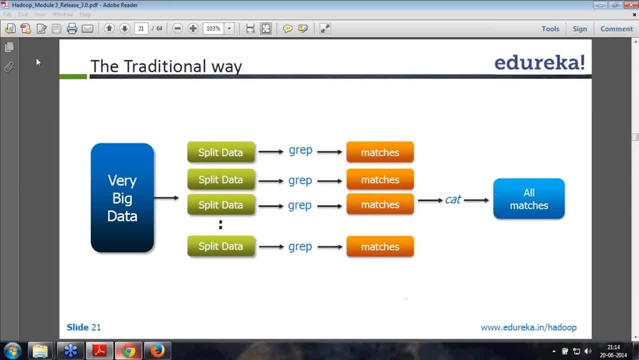 in a consolidated format. If you try to do it on your own, you have to do everything Shishabit was saying. what is grep? Grep is a Linux command which will go through the document to analyze something like a where class in a SQL query. 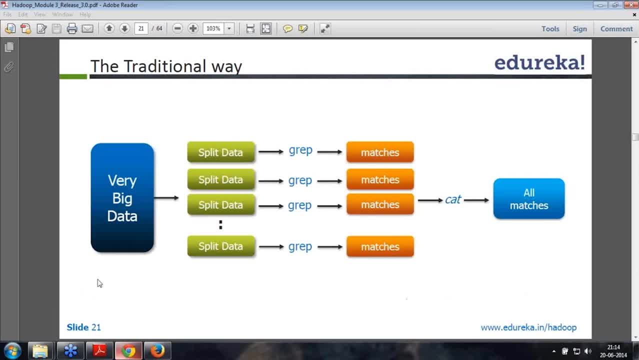 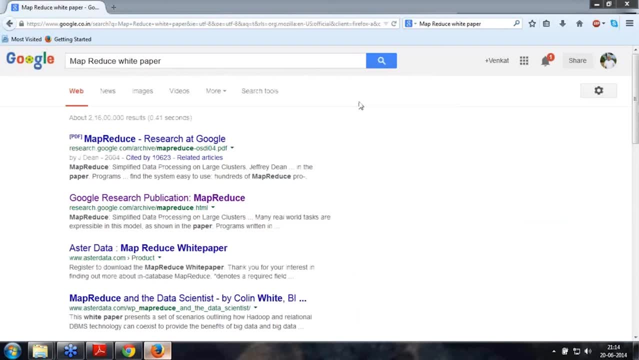 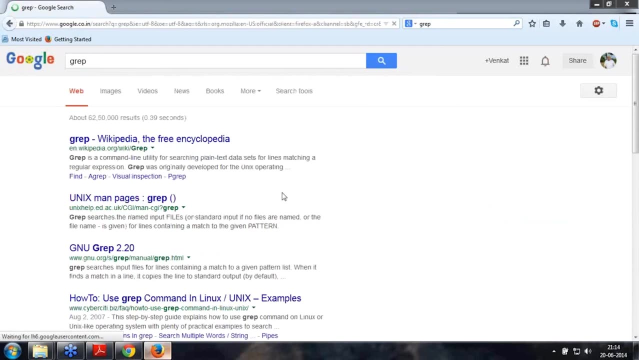 Cat is for displaying the contents or printing out the contents together. So these are two of the most commonly used Linux commands. So go down to Google. If you go down to grep and see grep, just press enter, you would see. there it is. 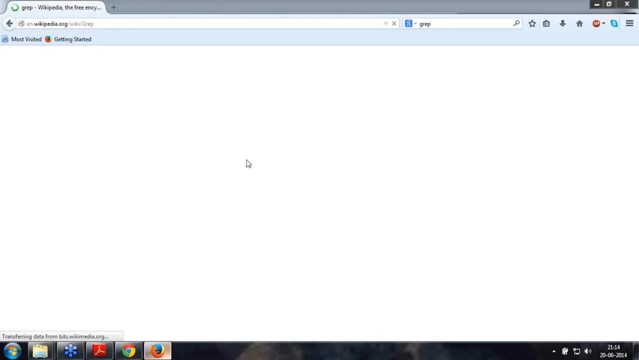 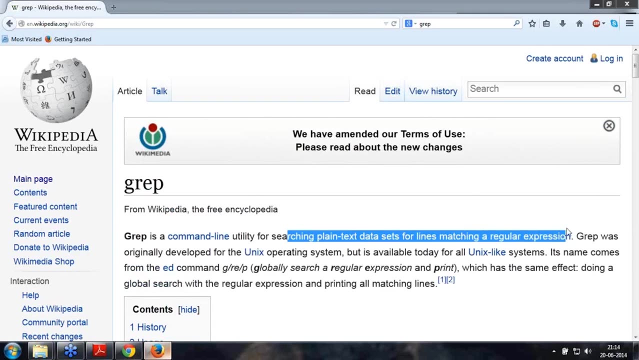 So look at the solution in the Wikipedia. It is loading up. So grep is a command line utility for searching plain text data for matching a regular expression. Okay, So grep was developed for Unix operating system but is available for Android. It is available for Android. 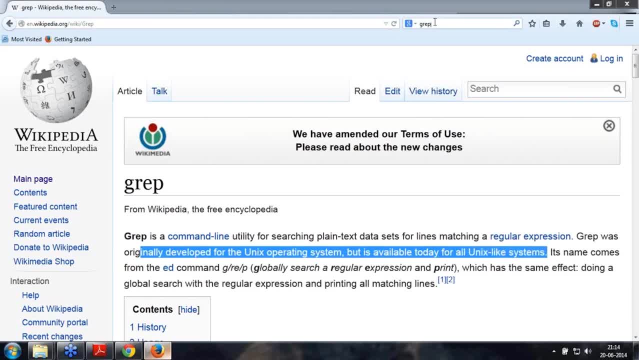 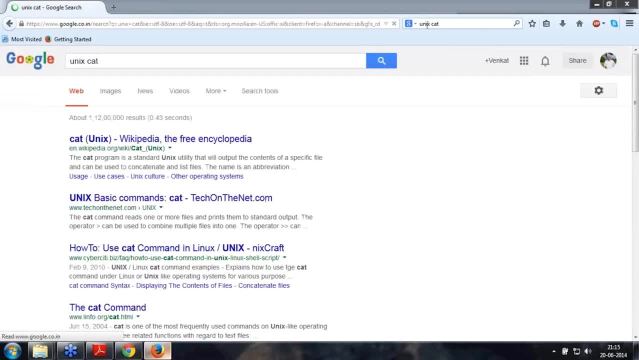 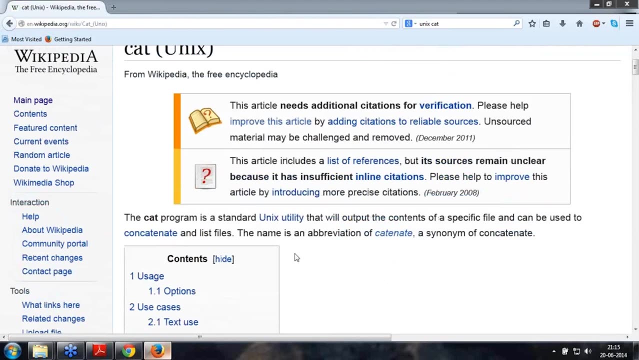 It is available for Android. It is available for all Unix-like systems. Okay, And if you talk about cat, all cats will come. That is the reason why I am searching for Unix cat. Okay, There we go. So if you look at cat, cat is. let it come up. 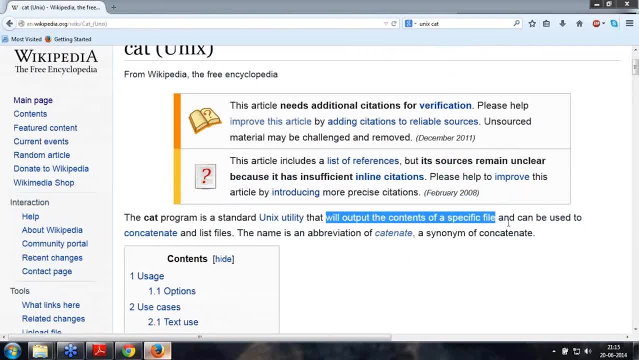 Yeah, there we go. So cat is a standard Unix utility which will output the contents of a specific file and can be used to concatenate and list files. Okay, So cat is an abbreviation of catenate or concatenate. That means add, Right. 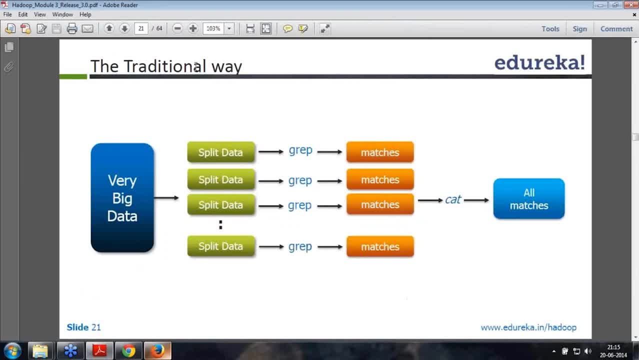 So these are all two Unix commands that we have, friends, So clear on that, Shishobit. So this is what you have to do, it in a traditional way. Okay, You're welcome. Okay, So now, there we go. 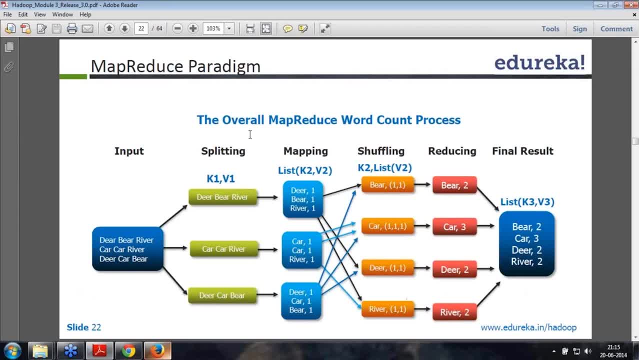 This is what is the MapReduce magic. So I'm going to spend about the next 15 minutes on this particular section. We have to be ready, We have to be crystal clear when we come out of this. Okay, So now imagine I have got a file that is going to be. let me open up my notepad and 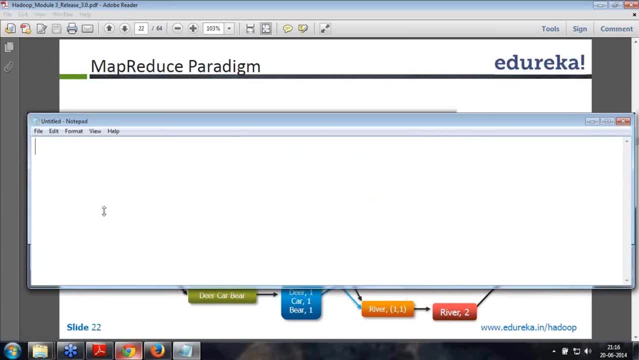 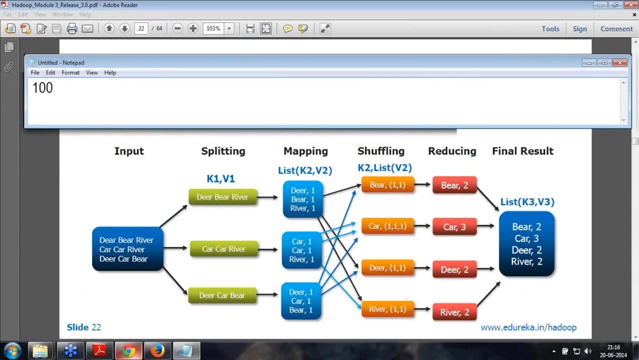 let me talk about the use case so that this becomes very clear for you. So let me put this up. Okay, So what am I having? I'm having 100 MB file 1 stored in the cluster in block, In blocks of 64 and 36 MB each. 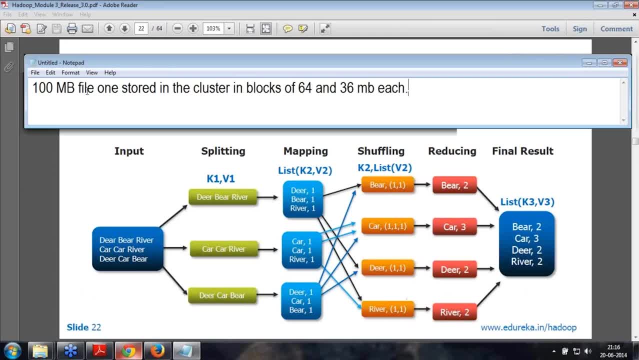 Fine, This is one of the example that you already have. Okay, So now, what am I showing over here in the input column? There are six columns that we are having. The input column is going to be the one block that I'm talking about. 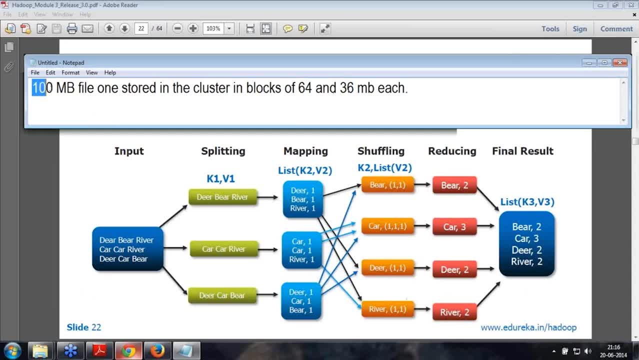 It could be 64.. If it is 200 MB, there will be multiple 64s and the balance- whatever 64 into 2- is 128.. So 364s and the balance of it. Right, Okay, So whatever might be the contents of a block- I am talking about one block over here. 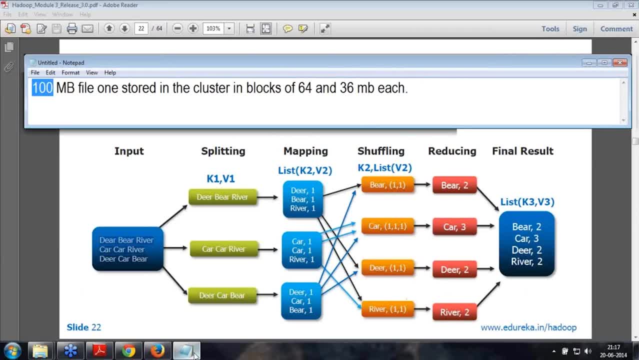 Fine, That's what I'm talking. The same thing would happen on all the blocks Parallelly. Because where are the blocks stored? Blocks are stored on multiple nodes, Right? I hope that is clear for you. In a real environment, blocks will be stored on multiple nodes. 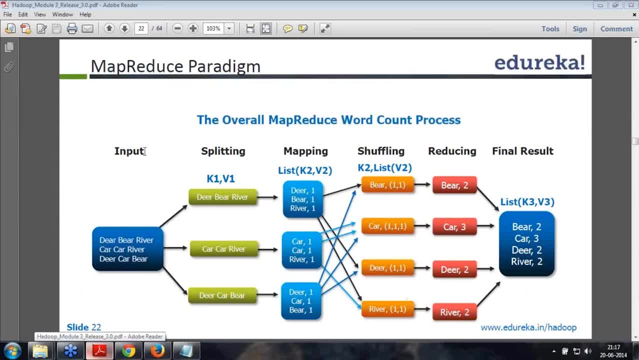 So the input over here is one block. Are we clear on this, guys? So apparently you are saying multiple data nodes. Yes, The blocks are stored on multiple data nodes, Right? If you are having 64 and 36, wouldn't the blocks be stored on multiple data nodes? 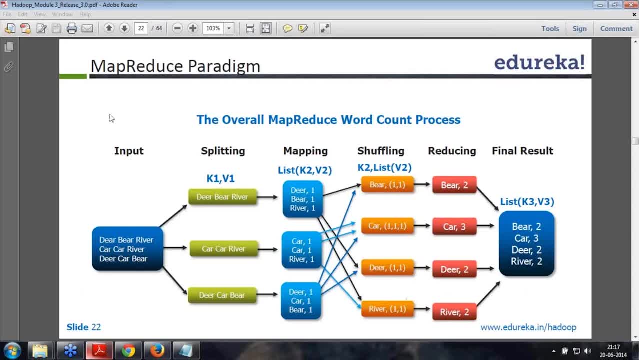 Right, friends, Good, So that is what is. I am talking about one block right now. Okay, Then remember, I told you something about input split. in our diagram, when we were doing the job tracker, 12 steps flow, I said there is something called as input split. 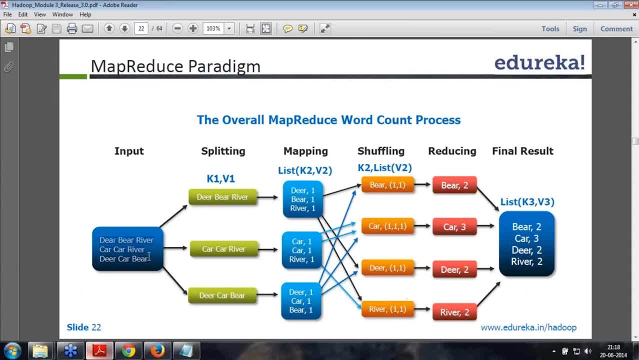 Right. So if this is the way how the data is going to be, we will have to decide how the split in logic would be done. Am I talking about block split? No, I am talking about record split over here. So we will have to tell the program, okay, how to look out for one record in that 64. 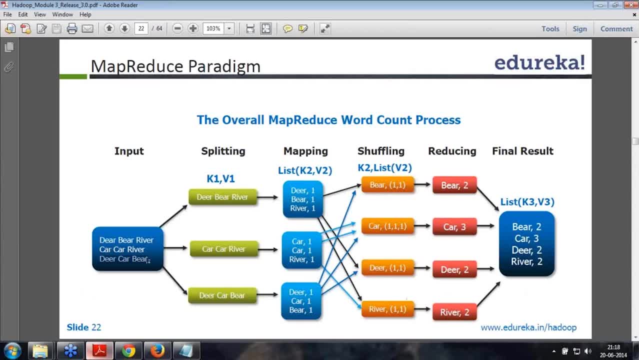 MB. And what is the default splitting logic? New line. So whenever you see a new line, it is considered as a new record. Okay, Exactly, Exactly. Actual data split is equal to record split in one block. Okay, Swapnil. 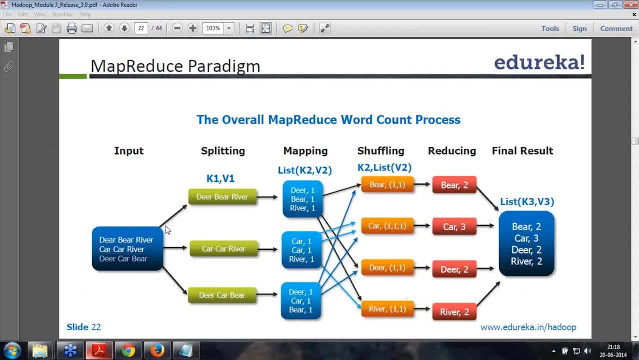 I am talking about one block. Remember I have got 64 and 36, two blocks separately Inside one block. I will have, you will have to identify a record. See if I am having three lines over here. hypothetically it could be three lines, it could be 30,000. 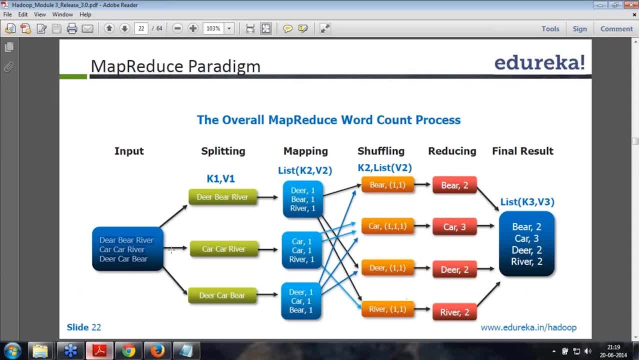 lines. it could be 3 million lines, Okay, Depending upon whatever the size of that 64 MB block. Okay, We will decide how to do the splitting. So there is a Java code which will be done. Exactly The same splitting logic will be done for the 64 MB and 36 MB, because they are one file. 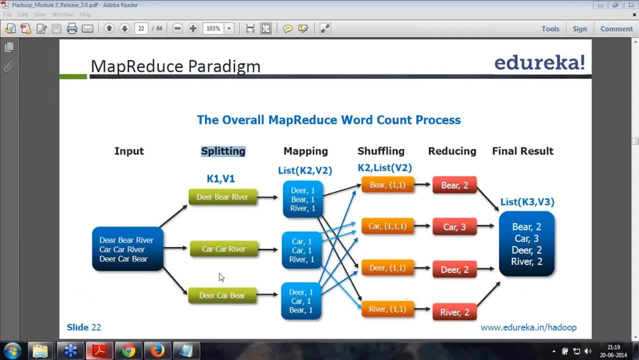 right. So you can't have a different splitting logic for one block and another splitting logic for another block of the same file. I hope that is clear for everybody. Please chip in in case if something is not clear. Okay, Fantastic, So this is how the splitting would be done. 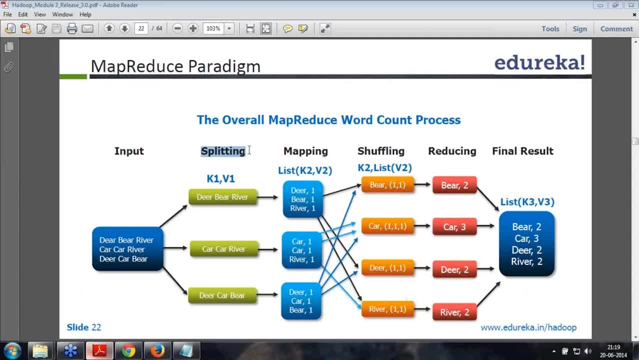 So what does the splitting do? here is let me tell you: when you do the splitting, okay, it converts a record into a key and a value, And that is what is going to be the input to the mapper. Please remember, the input and the output of the mapper is always going to be a key value. 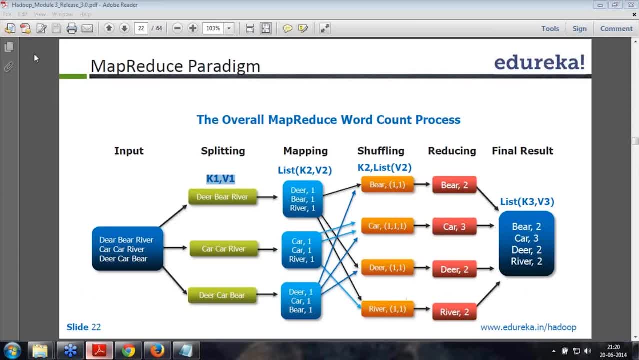 if you have read the definitive guide Properly saying Okay. So what is splitting? Give me an example of splitting. You can see over here, friend, This is an example of splitting. Am I not having three lines over here? Okay, 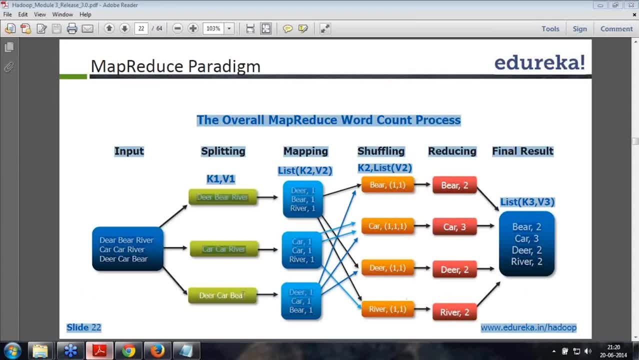 So how is it splitted? It is splitted into three separate records. I'll explain what are the key values, but then understand just this logic, friend. Okay, So what is going to be the key over here is the offset point. That means the position in the file is what is going to be the key. 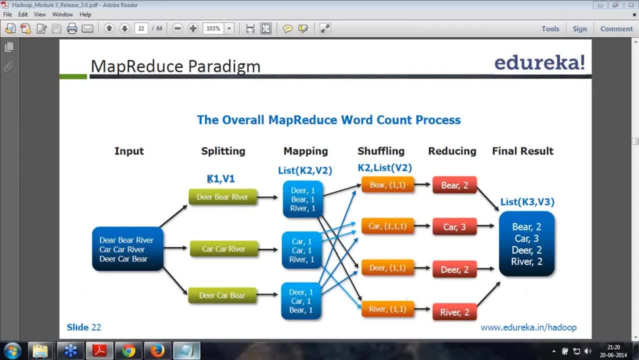 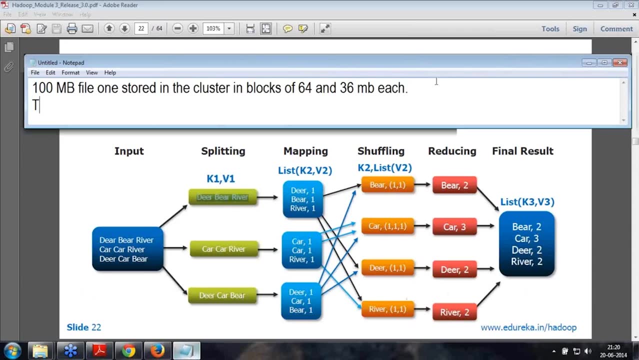 So is there the first line? Yeah, So the offset point or the position in the file will be zero for the first record. And what will be the value? The whole record will be the value. Okay, Let me explain that Okay. 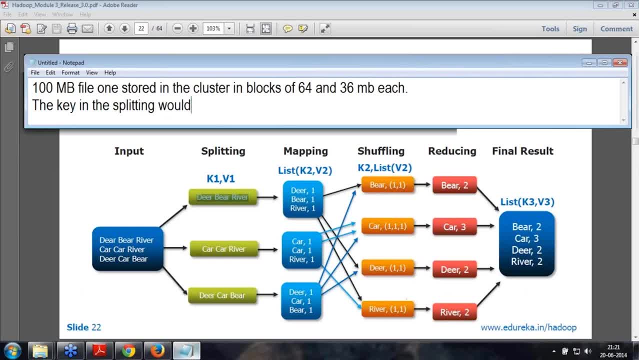 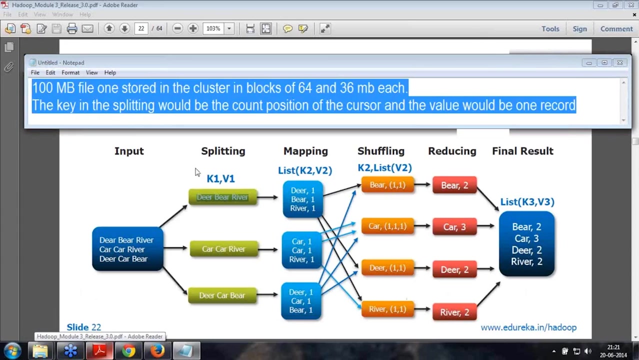 The key in the splitting would be the position of the cursor Okay Will be the count position of the cursor Okay, And the value would be one record Okay. So let me put this in the chat window for all of you so that this becomes very, very. 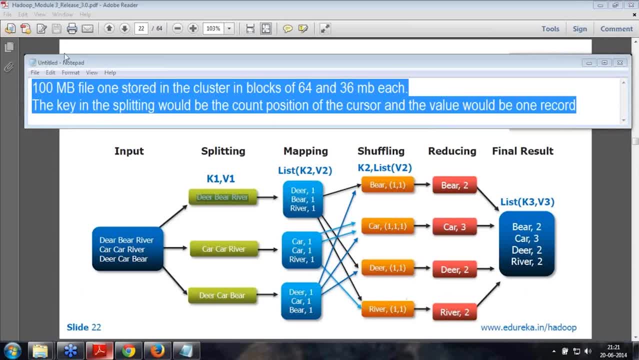 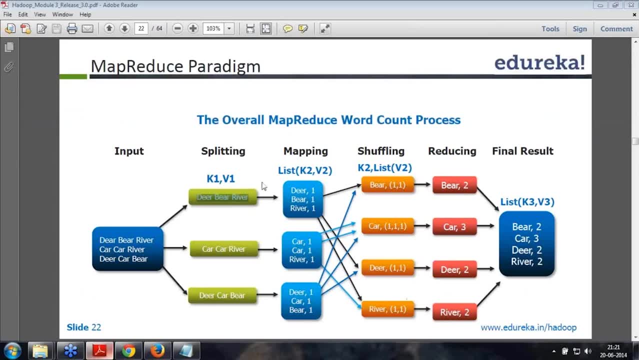 very clear. I'll explain multiple types of splitting also, Don't worry. Okay, So now if zero and Dear Bear River is for the first one, what do you think will be the key for the second record? Remember it is not zero. one, two, three. 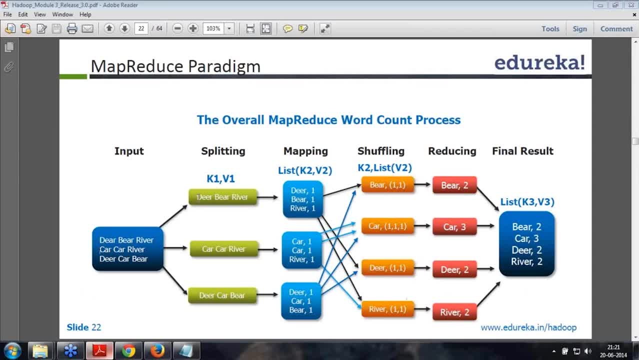 I'm not talking about the number of lines, I'm talking about the position in the file. So what will it do? It will do one, two, three, four, five, six, seven, eight, nine, 10,, 11,, 12,, 13,, 14,, 15.. 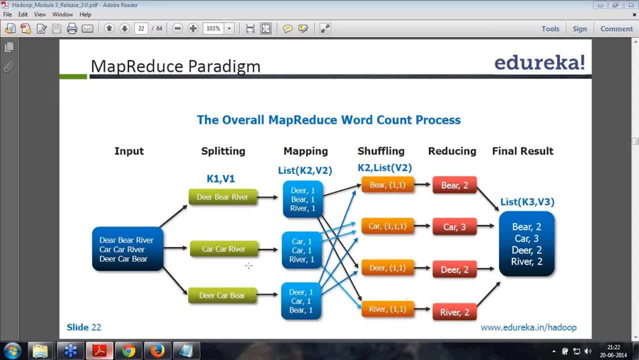 There are 15 positions. When it comes down to the next line, it will be 16.. So for the second record, the key would be 16.. Then 17,, 18,, 19,, 20,, including spaces. Okay, 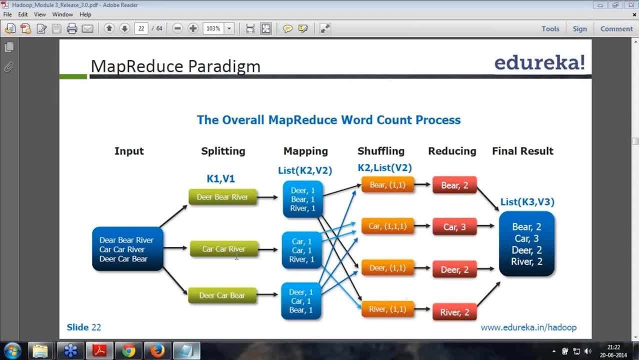 21,, 22,, 23,, 24,, 25,, 26,, 27,, 28,, 29.. And the third record will start with the key as 30.. And dear car beer. This is the way how splitting would happen parallelly at every record. 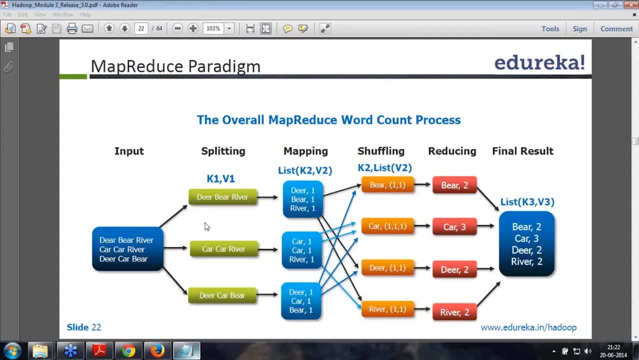 Hey, you only decide what is the splitting- Okay, And the split, the framework will ensure that it will give it a key and a value. You don't have to do any key and value, You just say how to split it Okay. 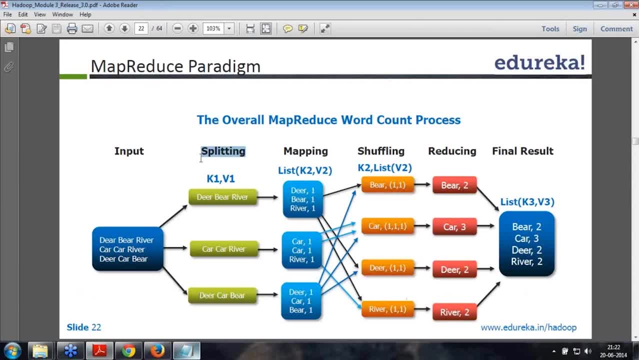 So how to split? it is based on a Java class. Okay, I'll be showing. Hey guys, you would also need- okay, next time, when I show you the API- the Hadoop documentation. Okay, Because I want to show you the documentation. 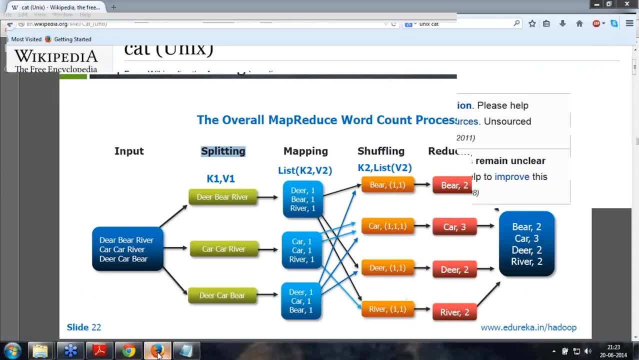 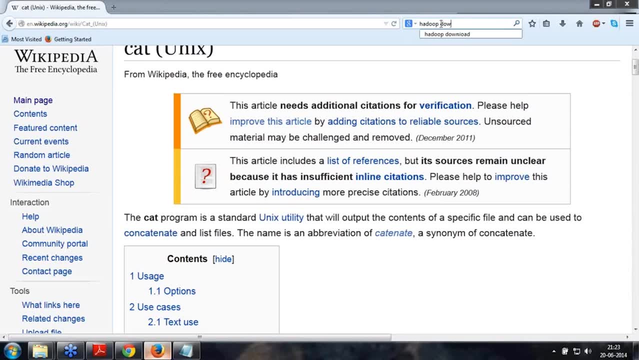 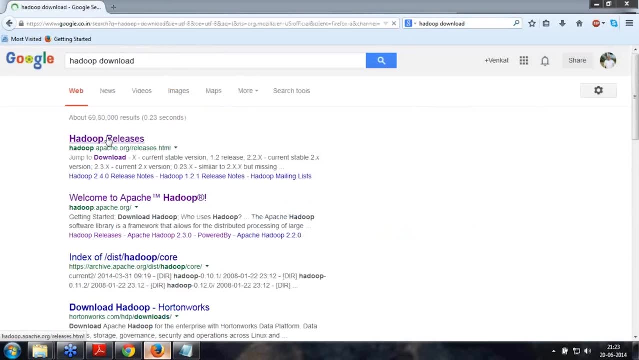 So on Monday I would need the Hadoop documentation. Let me show you from where to get it. So just go down to Google and say Hadoop download, Okay, And it will take you to Hadoop releases. When I click on Hadoop download, it will take you to Hadoop releases. 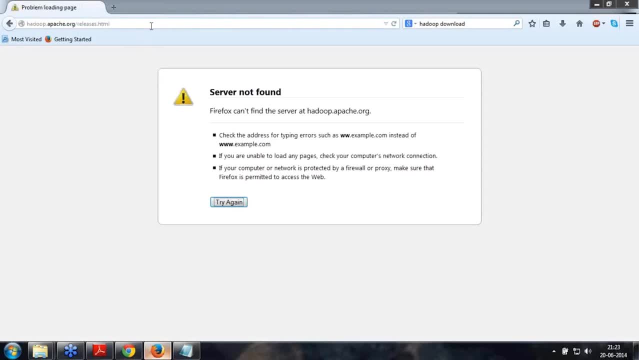 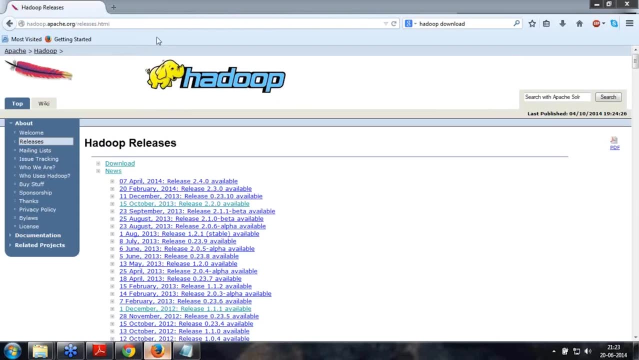 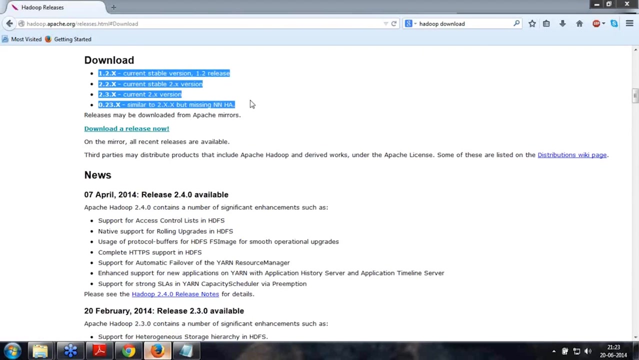 Click on Hadoop release And I will click on this. It will take you to a list of place where you can have downloads. So click on the download. And what are the major downloads you are having? 1.2x, 2x and 0.23x. 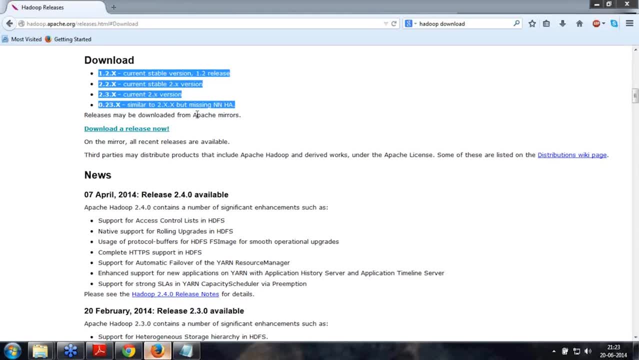 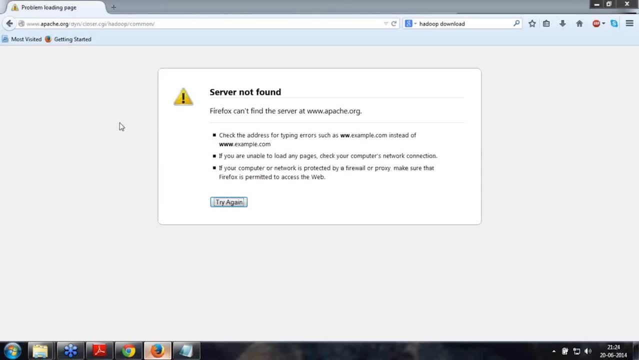 0.2x in fact. Okay, So click on download a release now. When I click on download a release now, you will see that it will take you to something very funny. in my machine I have to press enter once again for it to connect. 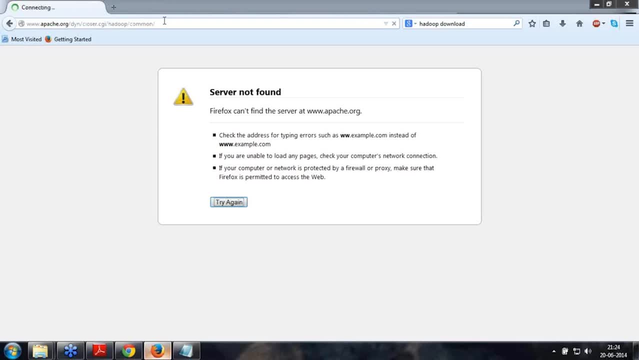 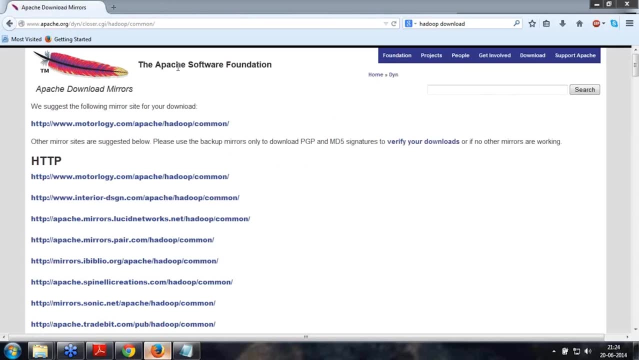 It will work. That is I need to look at. It only happens with my this thing, what I call internet. If I go down to a client place, it works fine. So, very funny. So when you click on this link, let me copy this link and give it to everybody. 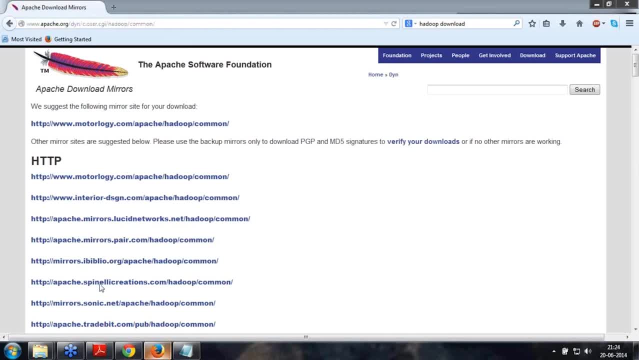 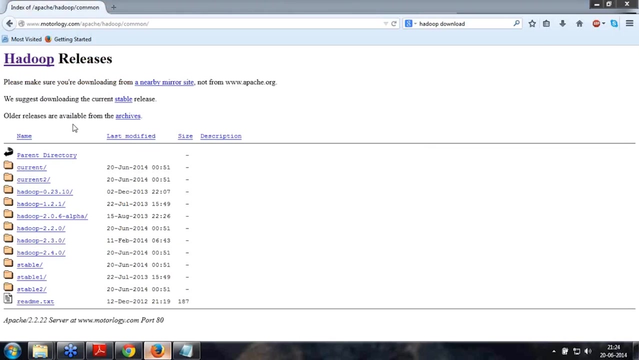 It will take you to a link. Okay, Swapnil says same problem for me too. Okay, So I am not the only one. Okay, Cool, So now let me continue. Hey, that's fine, That's good. So now, if you look at the link, there would be Apache would suggest a link for you, depending upon your geographic location. 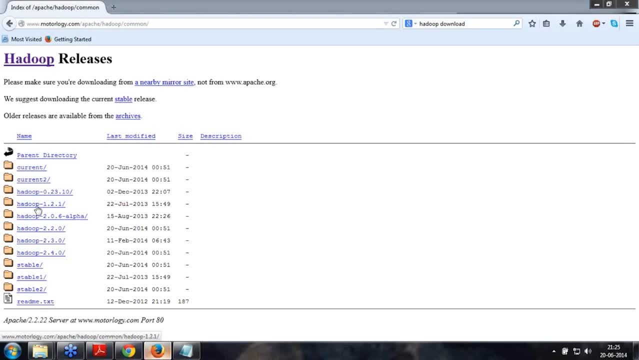 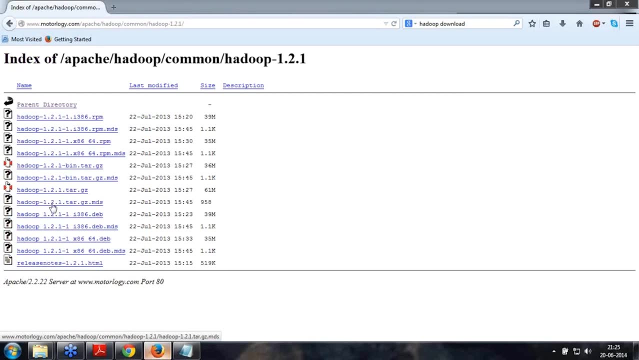 Look at your Hadoop: 1.2.1.. Okay, So when you click on this, 1.2.1.. Any release of Gen 1, and then you will have to download a file that is called as targz. Okay. 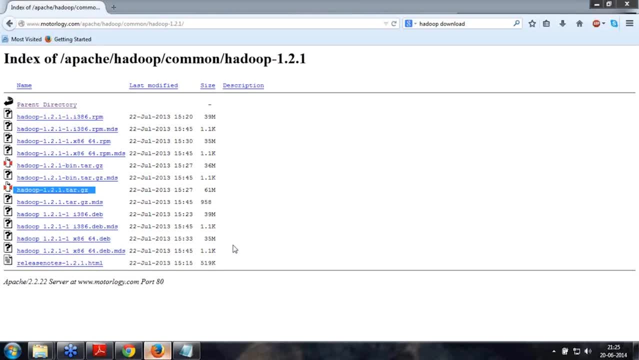 It's a 61MB file. Please have it downloaded and please have it unzipped. Using a RAR, you can unzip this targz file. Okay, friends, So the link, what I had given it to you: click on that particular link so that it will take. 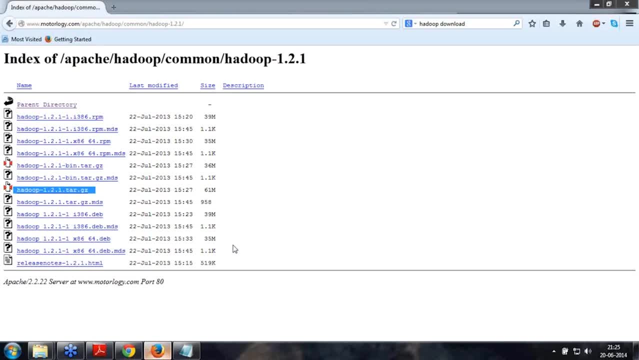 you to the location which is geography, Which is geographically closer to you. So see, this is how, like Hadoop, remember I told you, the name node will decide which is closest to you. So when you click on it, I am sure very few people will have got motorlogycom, because 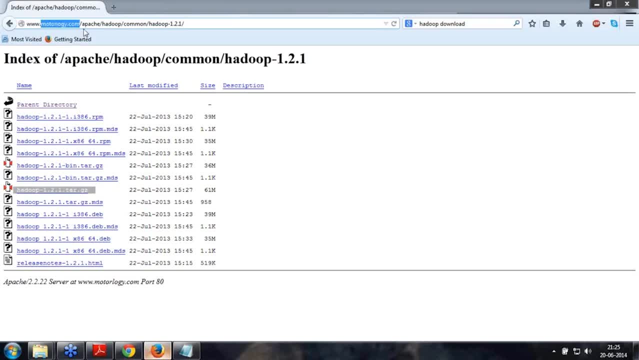 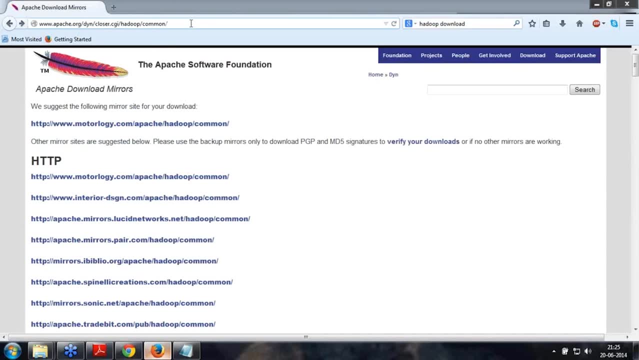 I am in Mumbai, So that is the reason why it has given me motorlogycom When you click on this common link. Okay, Just one sec. This is closercgihadoopcommon. Okay, When I click on this link, it will give you. 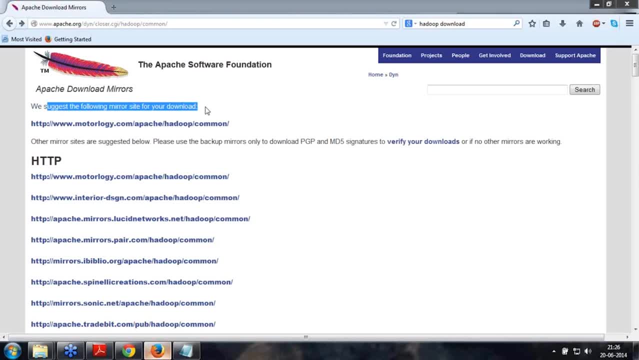 Okay, It will give you. We suggest the following mirror for your download would be based on your geographic location For the guys in US. I bet on it. you would not have got this, You would have got something else. Okay, So this is how the network proximity is done, even by Apache guys. 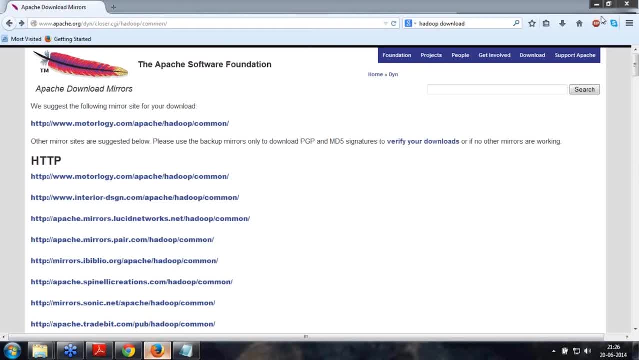 Right, friends. So once have your targz downloaded, extracted and you would see it Right, Very good. So Just one second, friends. Hey, hold on guys. Just one sec. Too many things at the same time, guys. 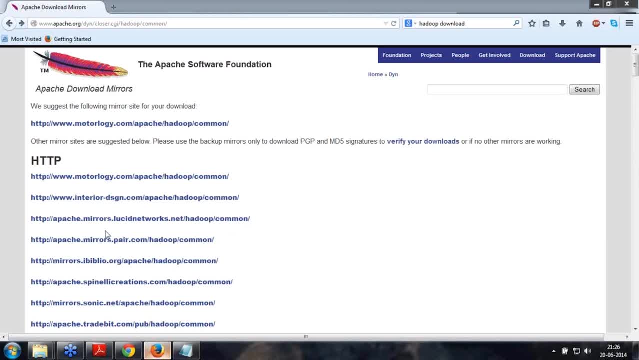 Yep, Yep, There we go. So, No, No, No, I am using a broadband. Okay, Shishabit said not for me. Shishabit has gone to Triviancom. is what Shrikant said. Everybody would be given a different link. 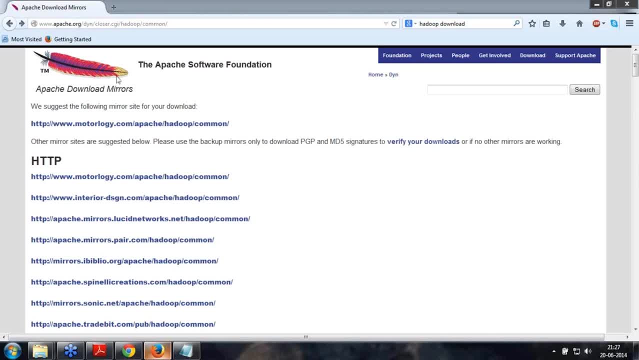 Don't worry. Okay, So, Shishabit, are you also getting the same link, Motorlogycom? Where are you based out of Shishabit? What's your location? No, I am not using Airtel. You are in Bangalore. 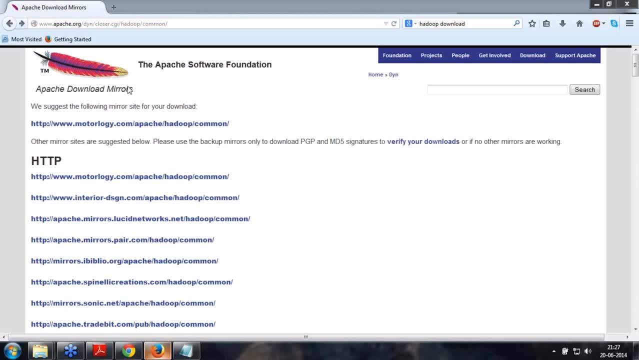 Okay, So maybe for the region, whole of the APG region, Indian region, they are giving you the same link. Okay, For others, like what Shrikant mentioned, He got another link, Cool, So No, I am using a fiberline Swapnal. 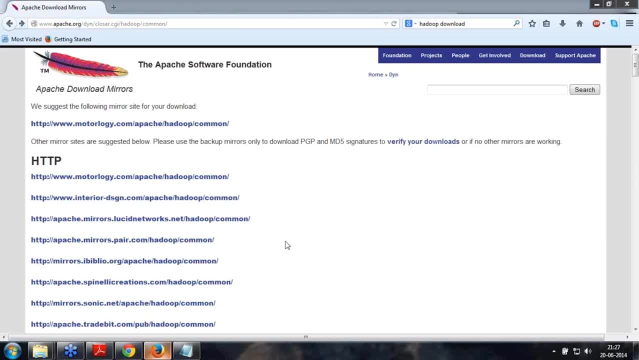 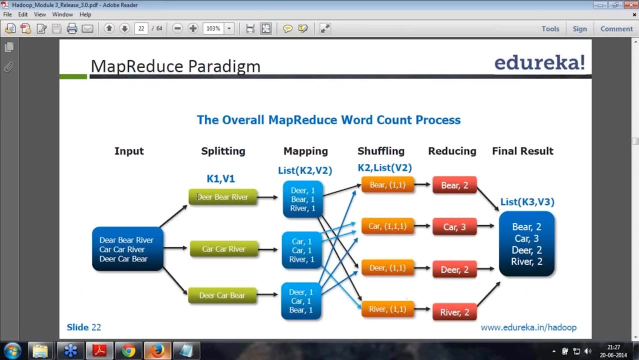 I am using MTNL, Fine folks, So let me minimize this. So now I hope we will specify what is the splitting logic, and the framework will convert it into a key and a value pair. The key will always be the primary, Okay. 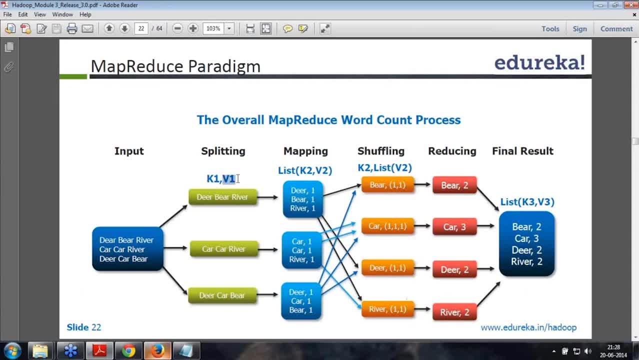 position in the file at the offset point and the value will be the whole record. Are we clear with the first two columns? So we need to be clear guys. right, friends? Any questions in the first two columns, The way how the splitting is. 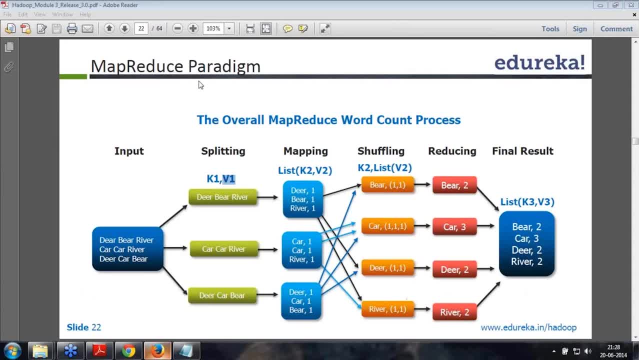 going to be happening is on all the blocks, wherever it is running. Good, Shishabit. I would really appreciate if others also. K1 is always a cursor position. That's correct. Hey, Ravi said splitting logic is based on space and new line. No, it is only going to be based on the new line Slash N, That is. 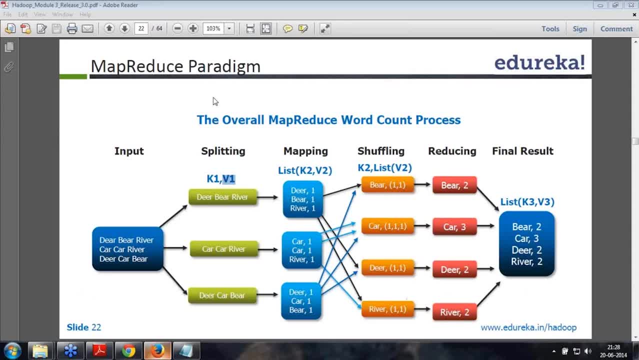 important. Ravi S Good, Upnikant, Fine, You are welcome. So now, whatever is the key value, irrespective of the data input, That's right. Swapnal Prapal, this is not for a word count, This is for any. 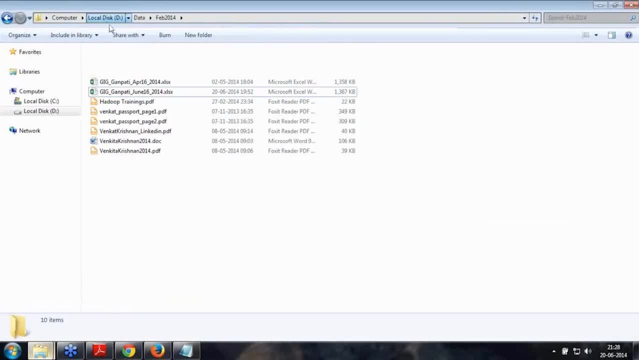 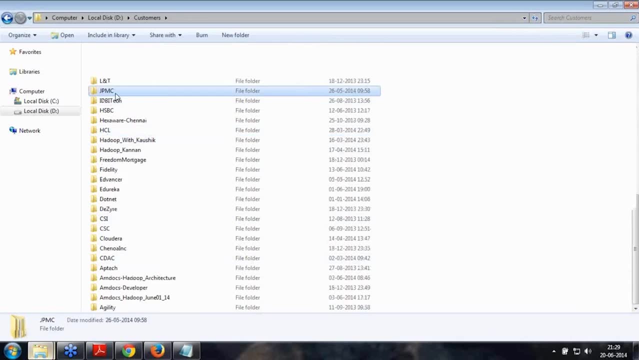 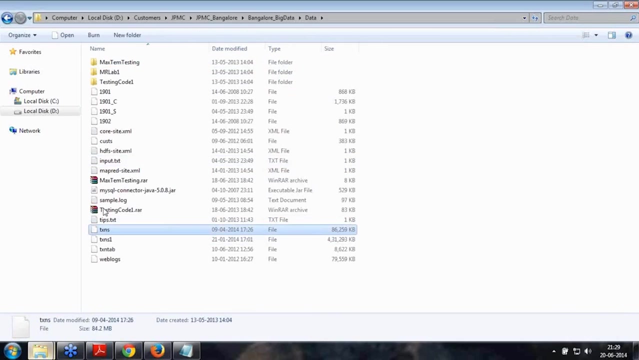 data set. Let me go ahead and show it to you. Let me go down to another example and show you a data set. Give me one sec. Let me go down to my JPMC and let me go down to the data. This is one data set that you will be seeing That is called. 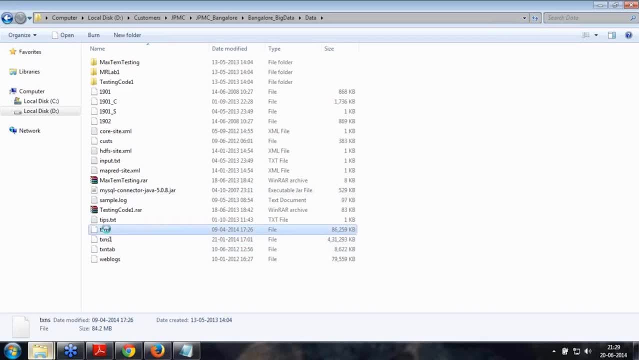 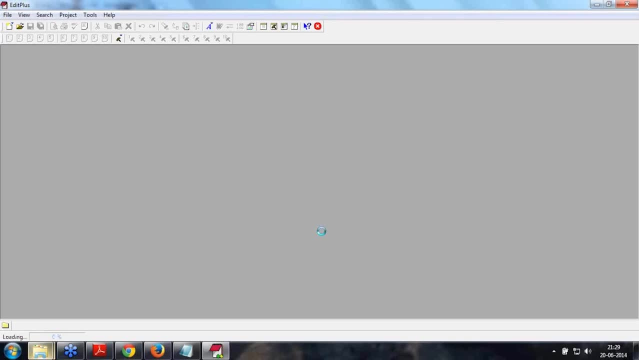 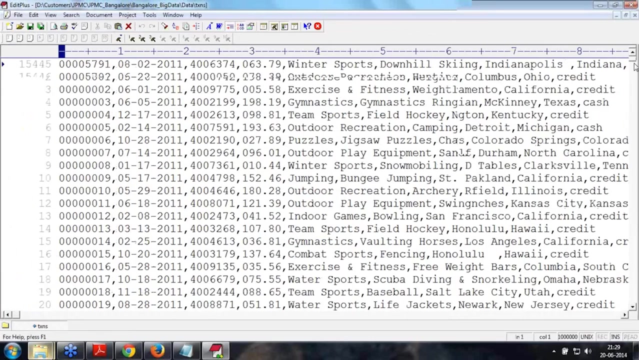 as TXNS, which has got one million records. So let me go down to that and open that in an editor. I think I've shown it to you earlier, I don't recollect, But then this is going to be one million records. Okay, So see over here You would. 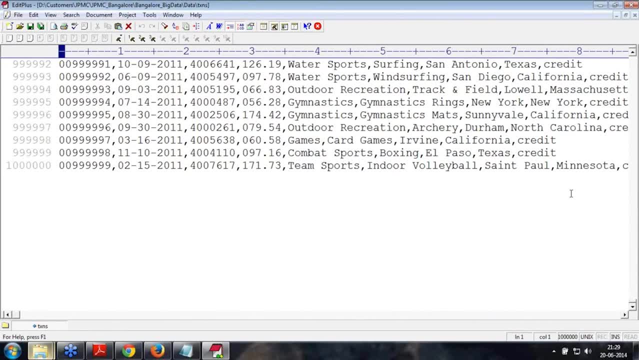 actually see one million records over here. So even for this one million records, also look at the 999,998 line. This is what is one record. Okay, Good, Upnikant, So I've shown this to you earlier, So that's right. 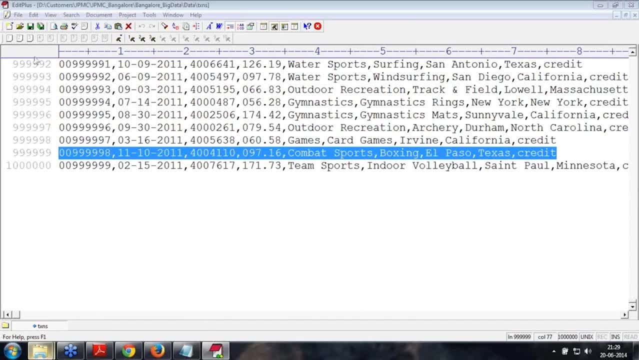 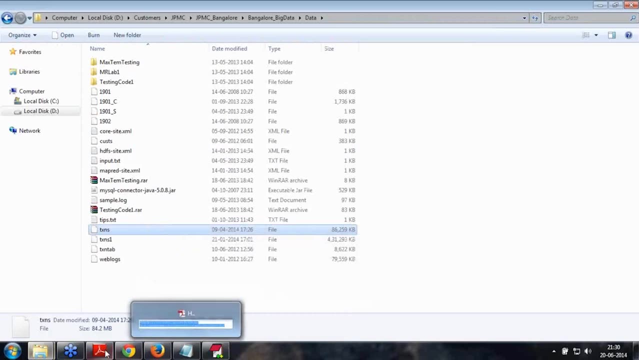 So this is going to be one record. So in most 95% of your structured data examples you would see this as one record. friends, Okay, A new line is always a record. Prapal, Make sense, friend, Let me minimize that. Okay, Cool, So now that is. 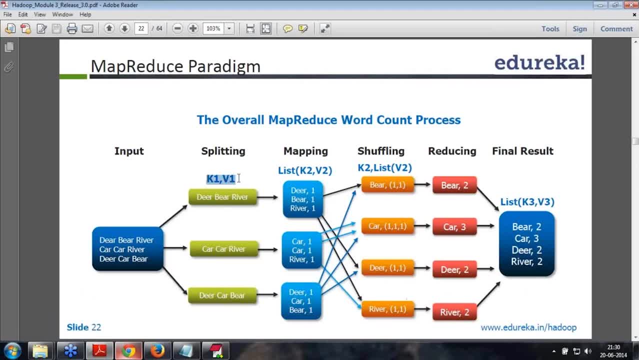 what is going to be inside the mapper K1V1.. That is key and value In the mapper. it's going to be K1V1.. So this is going to be K1V1.. So this is going to be. 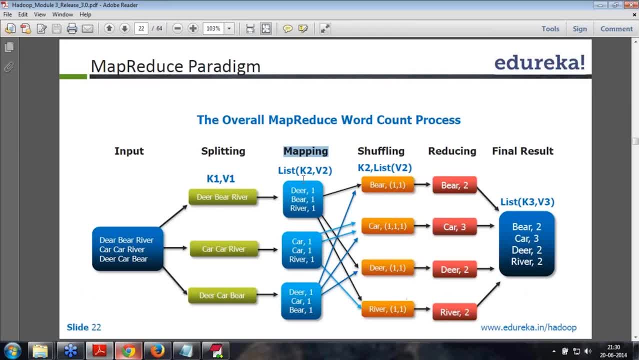 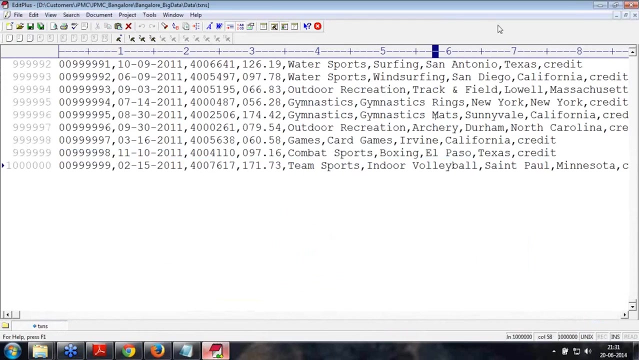 K1V1.. Okay, I will not show you the details- Two in the lower left right here to it- because I'm doing a word count. okay, in your transaction example, in your mapper, what will you do, supposing if I want to find out the sum of sales in? 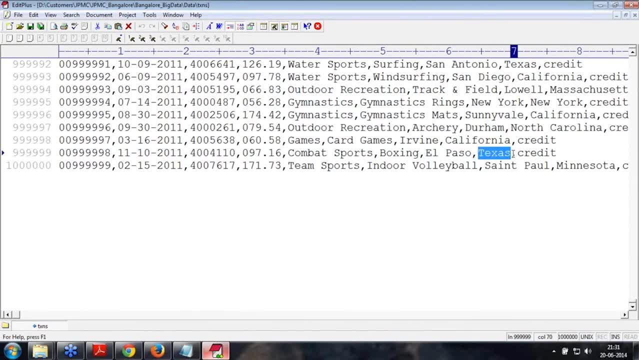 Texas. okay, I will in the mapper what will be the key and value. key will be an offset point and value will be the whole record. so from the record you will pick up two things. what are the two things you will picks up? you will pick up the. 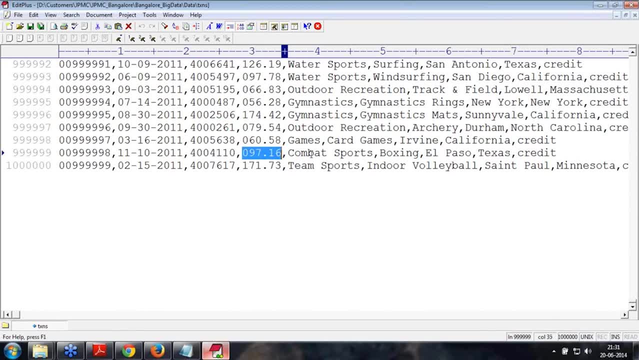 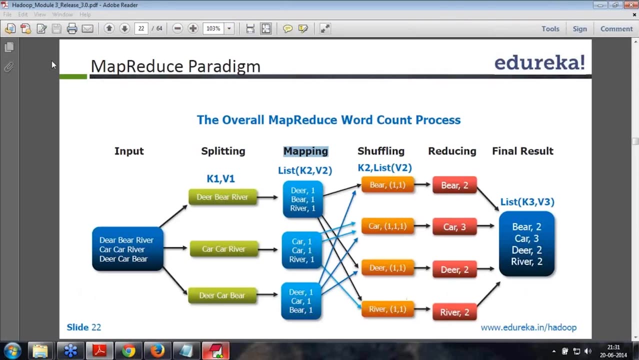 state and you'll pick up the amount. and if it is Texas, then only you will let the value come out of the mapper, because you are interested only in Texas, right? so that is what is the logic, what you will be doing it in the mapping phase. cool, so something was asking. so k1- v1 will always be an integer number, always. 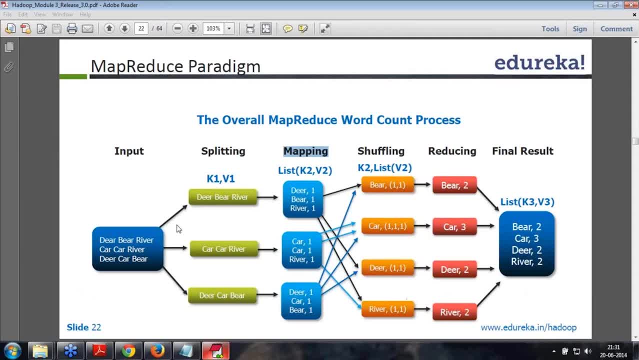 99.999999999999, 99.999999999999, counted for another hundred and hundred, five hundred and thousand four hundred and five and times. it will always be a long data type. it will be long because it won't be an integer. okay, so sign in. nabdi was asking me in java. okay, we are going to write the coding in java, right. 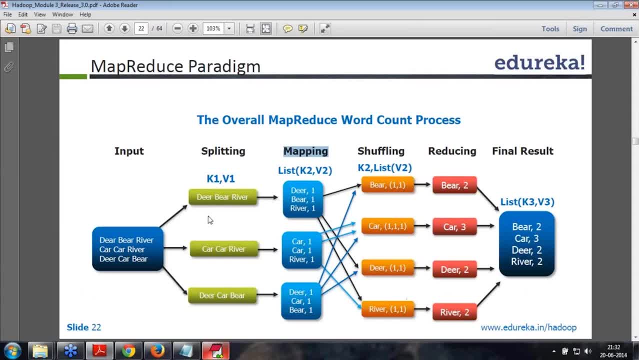 so what do we do? in the mapping you write your business logic of what you want to do. what are we trying to do? we are doing a word count over here, right? so i want to find out the number of unique words that we have and the count of the words. that is what my use case is about. so once 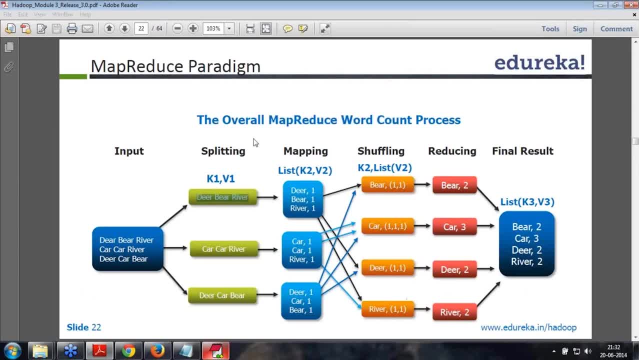 i get a record, what should i do for the records of now? i should break the record and suffix one to it, right? so the output of a mapper is also key and value. so that's the reason why you'll write the logic to break the record and the output would be a key. that is every record. 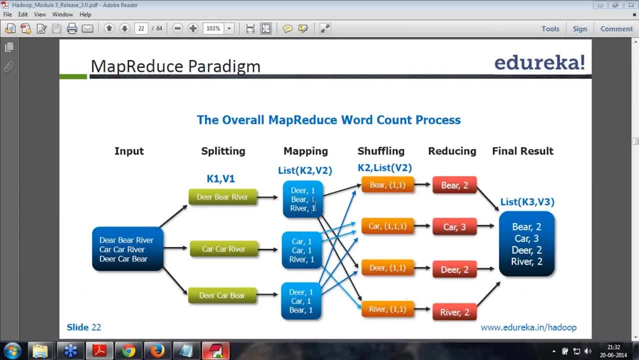 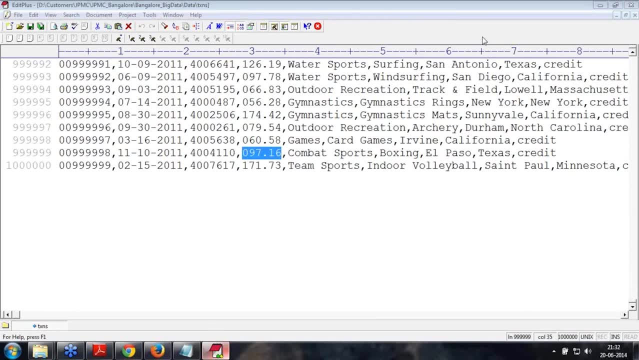 and to it it will always be one, because we want to just have the counterpoint of it in the example of your data set, of your transaction. what is my use case? sum of sales in texas. okay, so from one record, what am i interested? i'm interested in the state and the 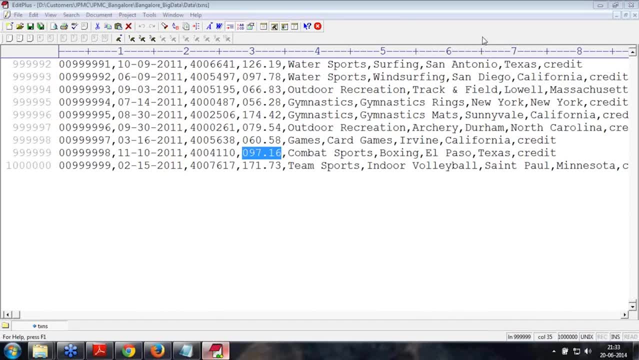 amount and when will i uh push out the- i mean what will come out of the mapper? only if it is texas, right. so i will write my business logic of what you want to retrieve from the mapper and what will come out of the mapper and what will come out of the mapper. 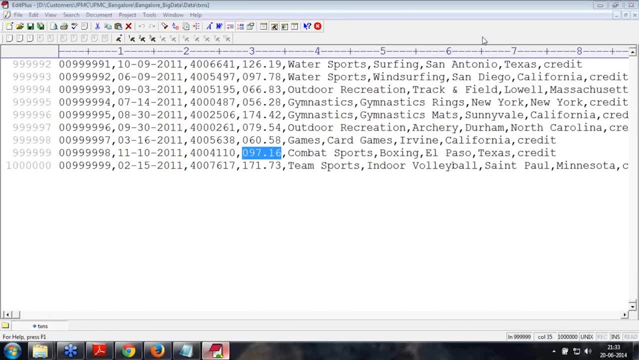 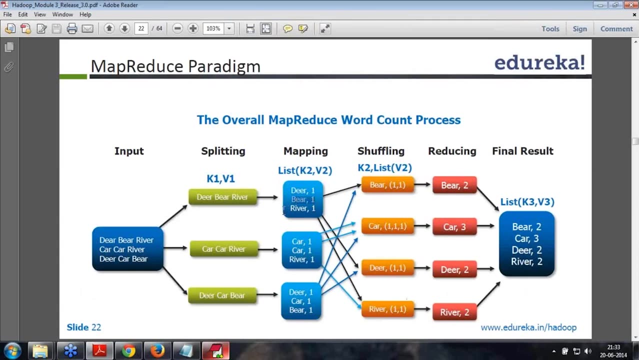 in the mapper. so the mapper will always- that's why it's called as a map. the map will always look at what do you want to get from the record. so in this case, the map will get the key value pair from the record. okay, so what will be the output of the mapper? it could be one key value pair or it could. 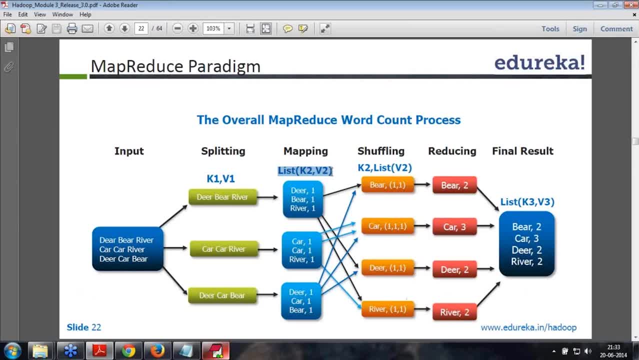 be a list of keys and values. list means more than one key value. in this example of word count you have got one more than one key value right. so in in another example of the transaction example, there was only one key and one value. make sense, friends. okay, very much soft null. 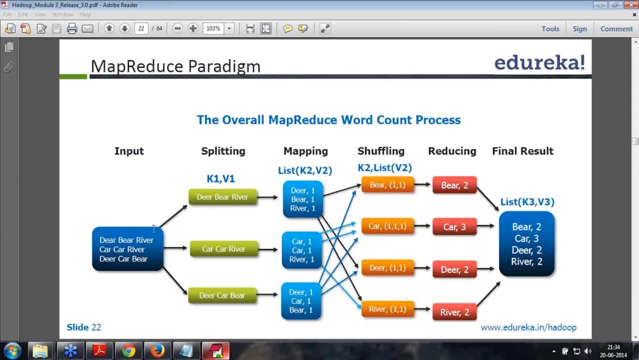 because you don't. you do a where clause select star from table name where. so when you do a where, doesn't that where apply to every record in your database? very much okay. so let me show you another example of a where clause select star from table name where. so when you do a where? 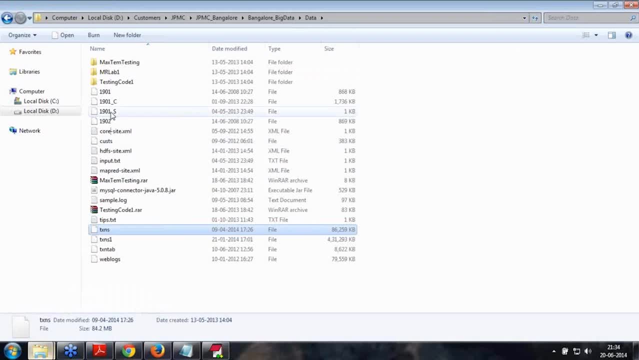 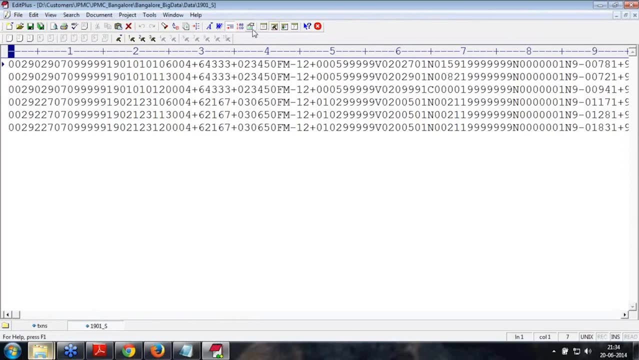 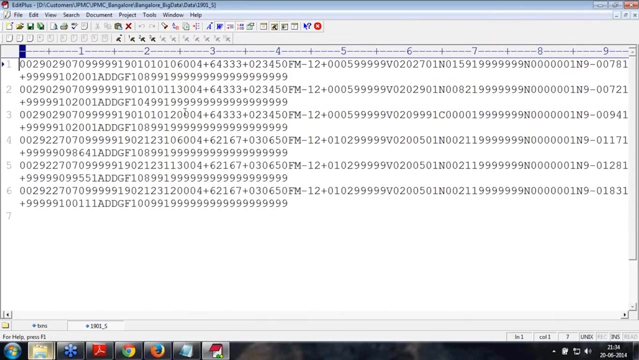 data set. so if you look at a transaction, a maximum temperature data set, okay. so what do you see over here is I have got six records. okay, and deliberately I'm going to do a word wrap so you can see this is how the data would be for those six records. okay, so what is needed over here is one record is a reading of a temperature. 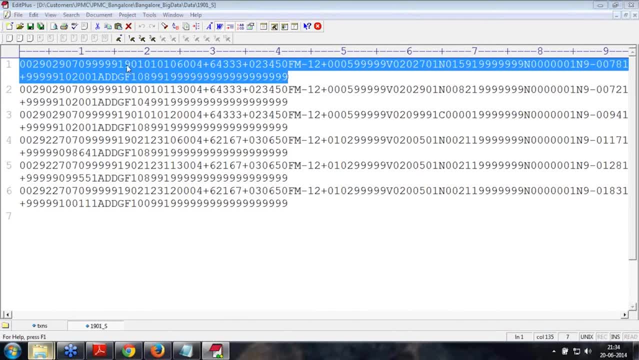 for a particular year and the temp. the year is going to be over here, okay, and the temperature is going to be over here. so there are fixed positions, right? so if I want to find out the max temperature per year, I will have to find out the temperature and the year. so what will be the key? key would be: 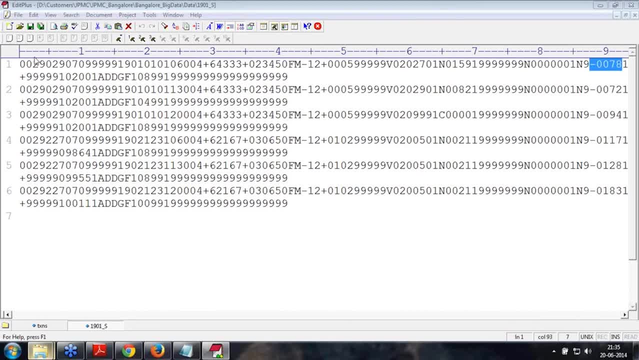 the year and what will be the value. value will be the temperature. whatever you want to do to do the aggregation on fine, Fine. So that is the way how you'll have to start looking at it. Everything is going to be a key-value pair and we'll have to understand that very clearly. 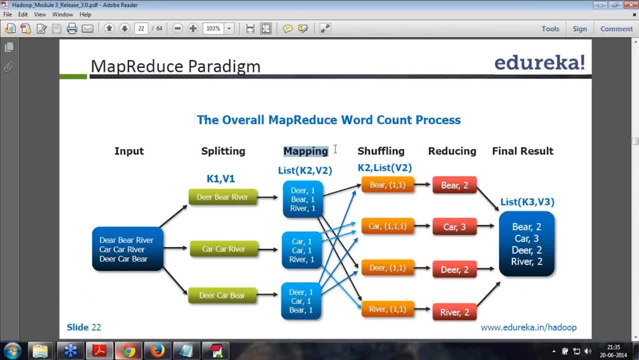 Cool. So that is what is the output of the mapper: a key and a value. So now the first three steps are going to be done on every node, wherever the data is going to be. Okay, Hope that is very clear with you. 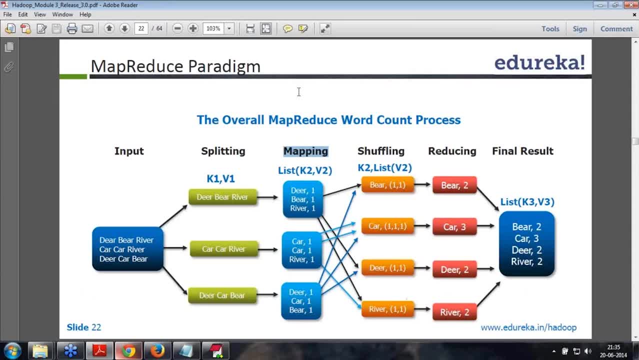 It is going to be done on every node, wherever the data is going to be. Then what do you do Whenever the mapper finishes? okay, where is the output stored? guys? Shishabit was asking: what is K2?? K2 is what is the output of the map. 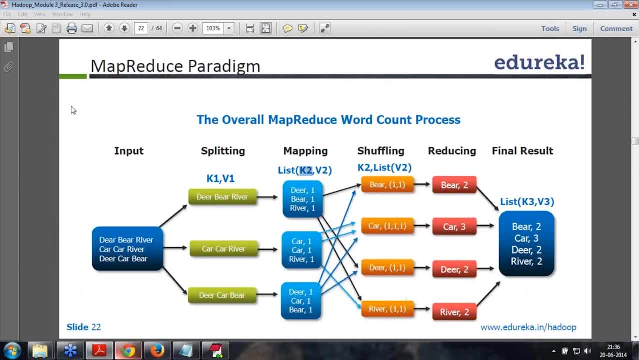 So you have to identify from a record what is a key and a value. right, So identify what is a key and a value. So what is a key that is going to be There from the record that you want? So in the example of the word count, it will be the word. 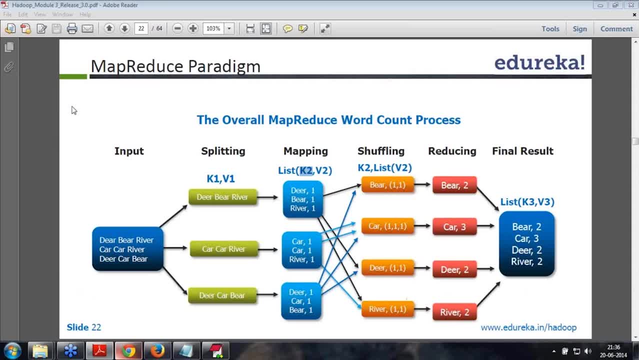 In the example of the transaction data set, it will be the state. In the example of the max temperature for a year, the key will be the year. Okay, Good, good, So proper two seconds. I'll explain that. So Swapnil was saying what I understood is that we have to go through the record manually at start. 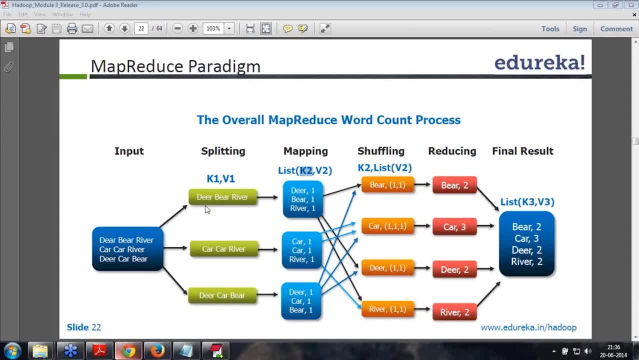 You'll have to pass on the data set to the record and the framework will ensure So. we should have going through the record based on the new line. We don't have to worry about it, It's the responsibility of the framework for doing that, Swapnil. 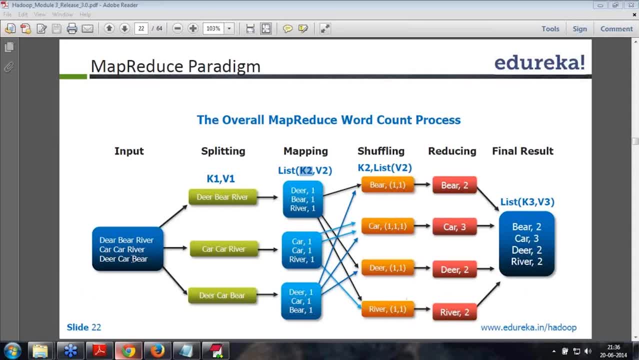 Cool Papal was asking: in case of unstructured data, how is the splitting done? In case of unstructured data, also like a log or like a blog, you will have to decide the splitting logic. In the case of a log, it could still be one line, but then, since it is semi-structured, 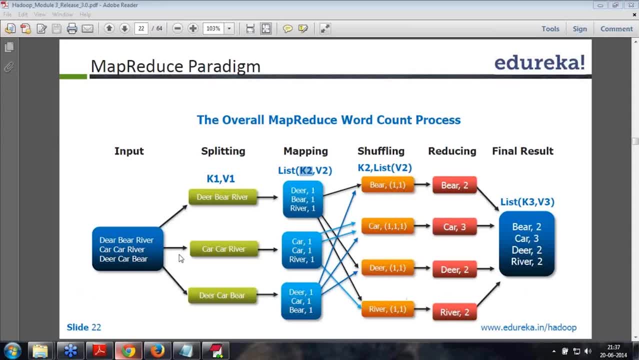 you will have to use regular expressions to get what you want from the log. Okay, In case of audio-video images, one file will be one record, So you have to identify the splitting logic properly. Cool, Fantastic, Srikanth has said it is just like a typical word count example using a hash map, right? 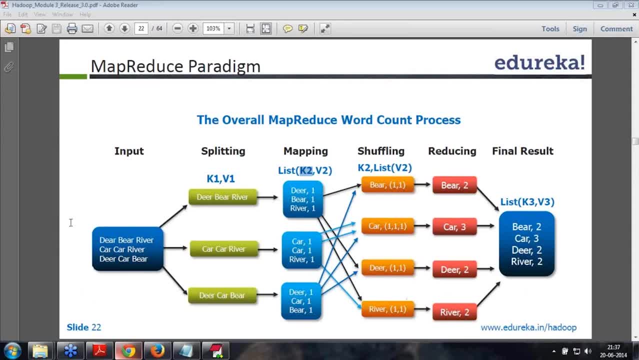 Very much Okay, So that's a very good analogy. Cool, Okay, Okay, Okay. So then Ravi was saying why car in the second is not showing car to? Why should it show car to Ravi? 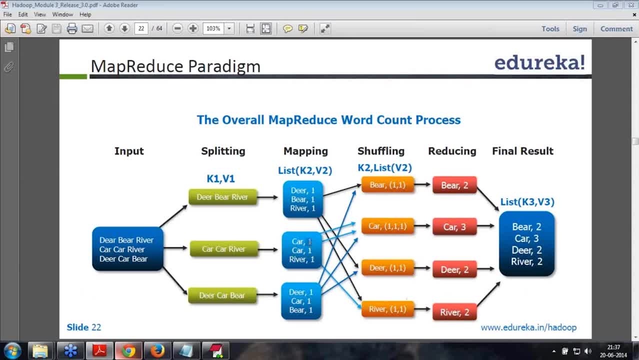 Because you are going through every word and suffixing one to it. You are not doing a business logic to see if there is already a key present and then I should add one to it. You are not doing that in the mapper right. The mapper is going to be a code which will look at, split that words and then write one to it. 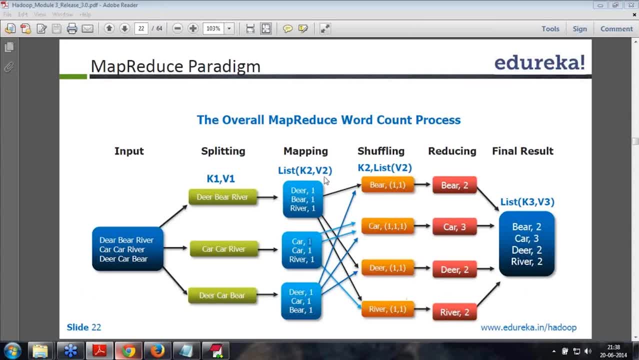 That's all the mapper is doing. If you want to do some addition, If you want to do some additional logic, then you will have to build in the code. Fine, Cool, Ravi, Very good problem. So the first three columns are going to be done in your every mapper node where the data is. 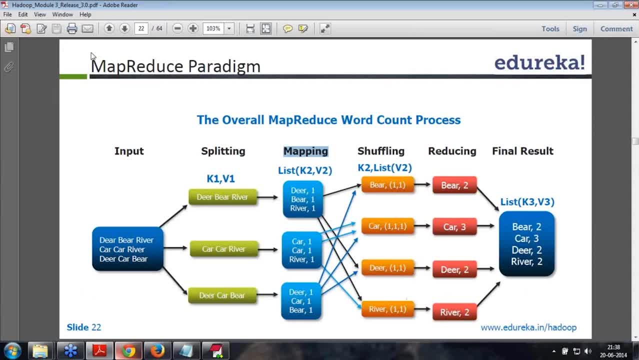 So now tell me, where will the output of the mapper be stored? Yesterday we did some configurations right In the mapper-sitexml. Where do you think is the output of the mapper For stored folks? I'm acting like Annie now. 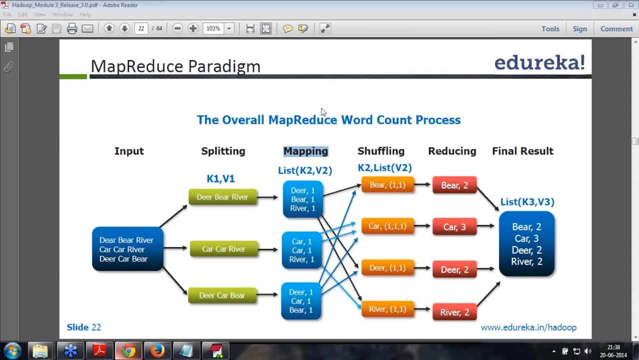 Okay, No, no, no. The final output is what is stored in HDFS. The output of the mapper is not stored in HDFS. Yes, Yes, Yesterday we had a property called as localdir, right in mapperetxml, right. so in mapperetxml there was a location. 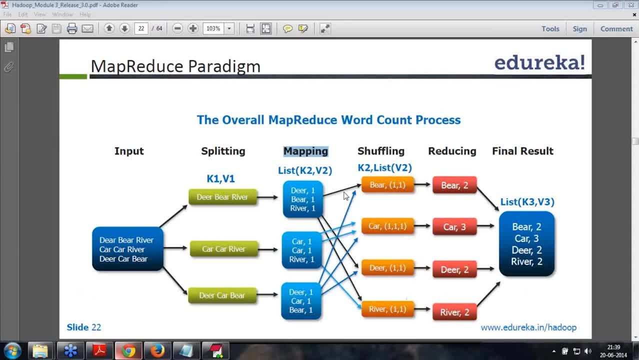 called as localdir. it will always be stored in the local file system of the node. okay, it will be stored in the local directory wherever your location of localdir. remember, I told you two things yesterday: localdir and systemdir. systemdirectory and localdirectory. 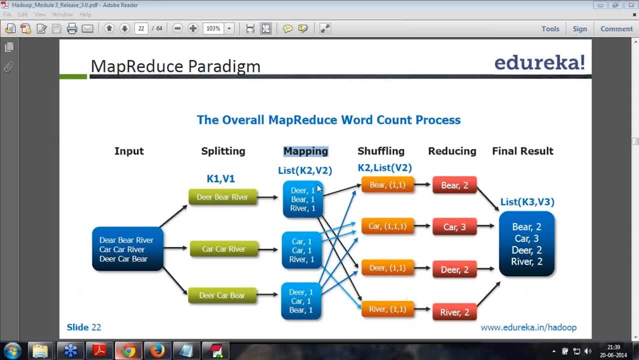 wherever your localdirectory directory location is mentioned, the data will be stored over there. friends, okay, perfect. so now, once one of the mapper is finished, okay, there is something called as shuffling. that is going to happen. so who is going to orchestrate? 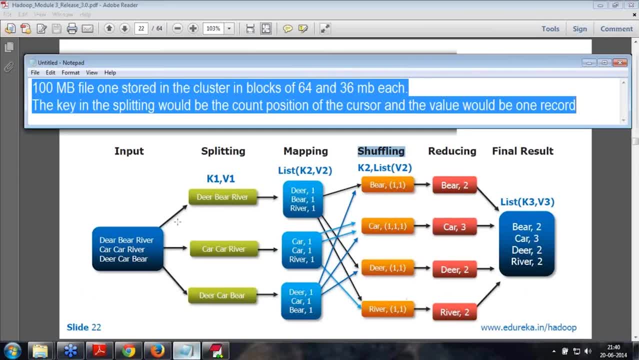 the shuffling. It is going to be the master. so let me go ahead and explain that shuffling is going to be controlled by the master of mapperadios. that is going to be the job tracker. okay, so what will the job tracker do? here is the movement. it sees that one of the mapper is. 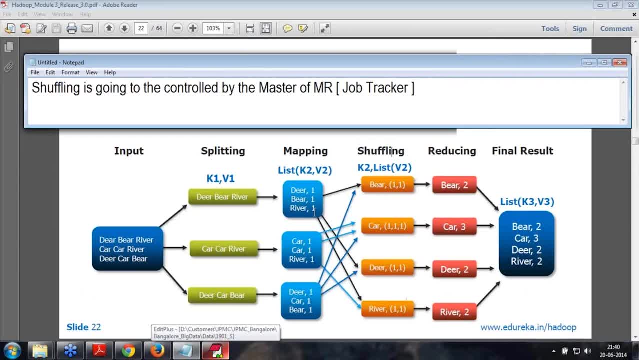 finished. okay, it will assign a separate partition In which it will give it to a reducer slot. okay, let me write it down. okay, the job tracker will assign a separate partition. so how do I decide the partition? okay, that. 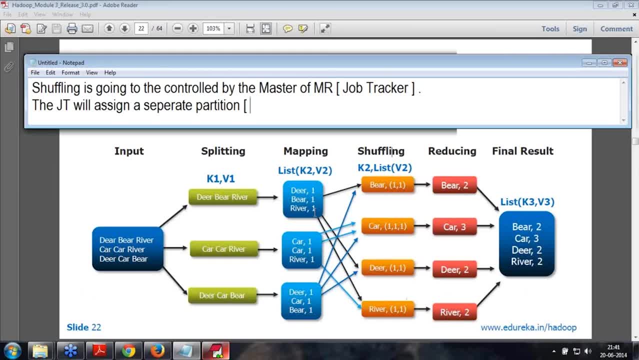 means separate area, okay, or separate collection. you can say, okay, will assign a separate partition. okay, what is a partition? How do I select the partition? Default partition is the hash of the key. okay, it will assign a separate partition. 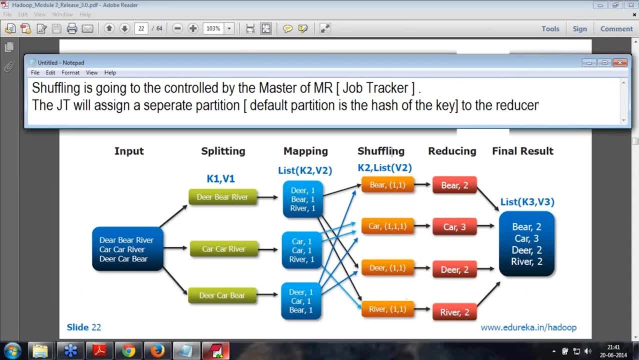 to the reducer, to a reducer slot, to a reducer slot. okay, what is a reducer slot, A reducer? I should say a reducer instead of a slot, a reducer, okay. so now I am going to go ahead and copy this for you. 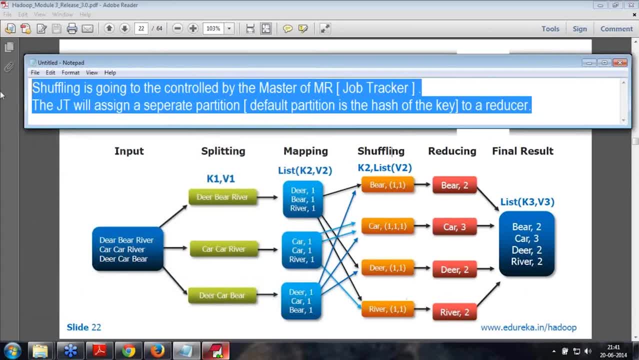 Guys, just one sec. by mistake, I did control S, so let me do a copy paste and put this in the chat window. okay, so just one sec. Okay, got an SMS, so I just saw what the SMS is. that's the reason I got distracted. 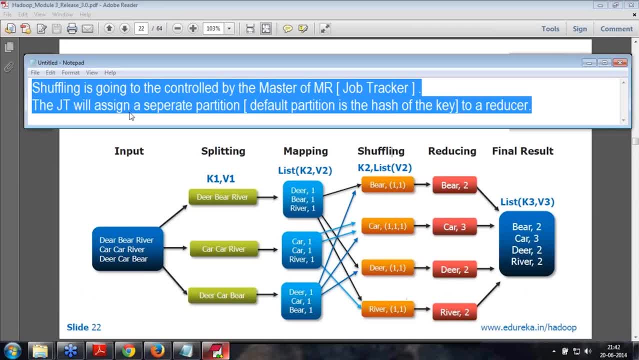 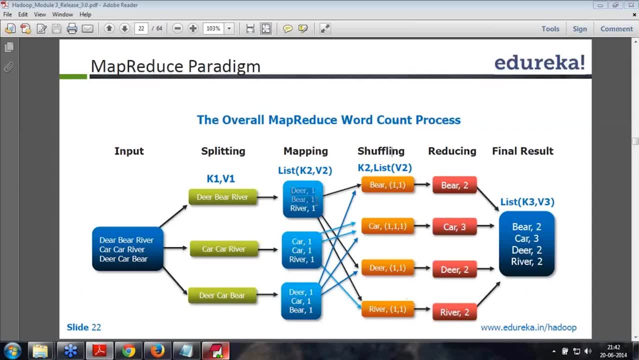 let me do a control V and that is sent to all. So let me look at this, guys. so whenever one mapper is finished, the shuffler will. that means the job tracker will start the shuffling process, so it will assign a dir. that means 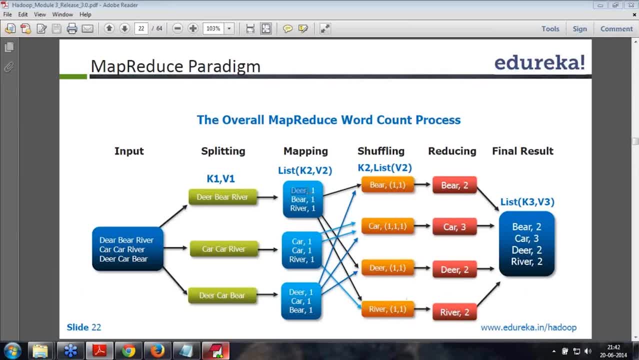 it will look at the hash of the key, Okay, Okay, So the reducer slot. you are responsible for this. So which is the reducer slot it's assigning? It's assigning dir to it. okay, this is the first reducer slot. so what it has done over? 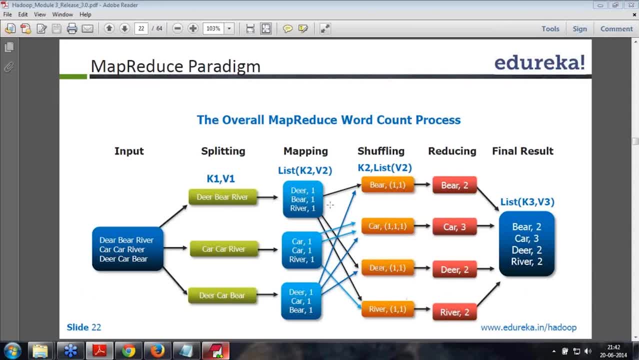 here is: it has taken the key, okay, and it has given the value also to that particular reducer slot. Then bir bir comes down to another reducer slot. river is another unique value. that's why it will go down to the another reducer slot. 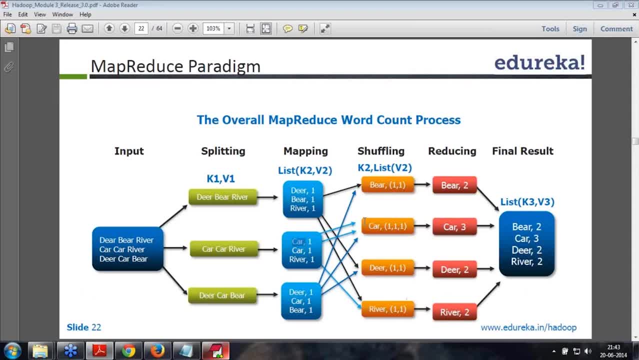 Then when the second mapper finishes, car is another unique slot, so that's why it will go down to another partition. now, car is already there. that's why the second value will go down to the second partition. river is already there, that's why the second value will go. 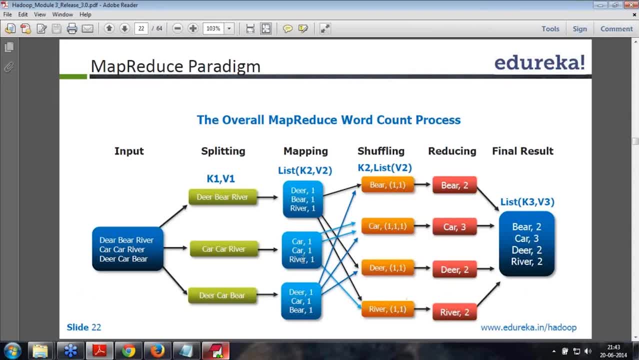 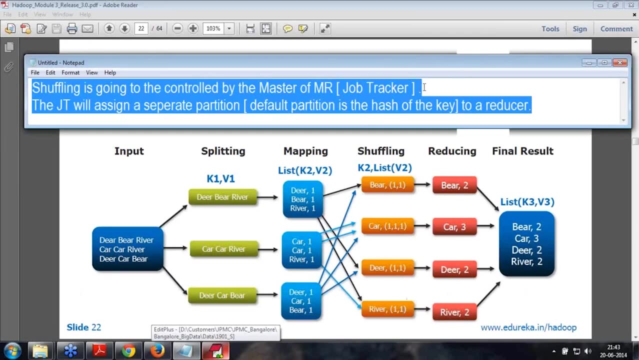 down to the same partition which had the river, the first river, then same way for dir, car and bir. So what happens over here is the shuffling process is going to be orchestrated by the, orchestrated by or controlled by the master of MapReduce, that is, JobTracker. so as and 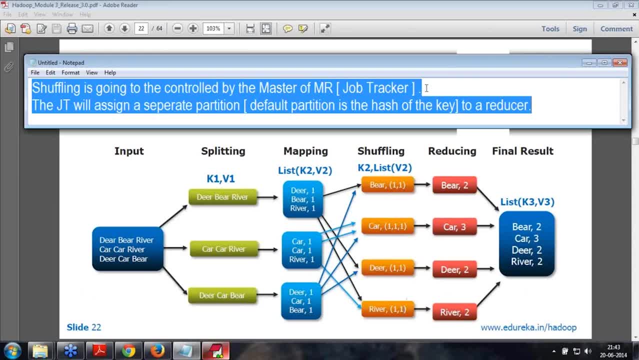 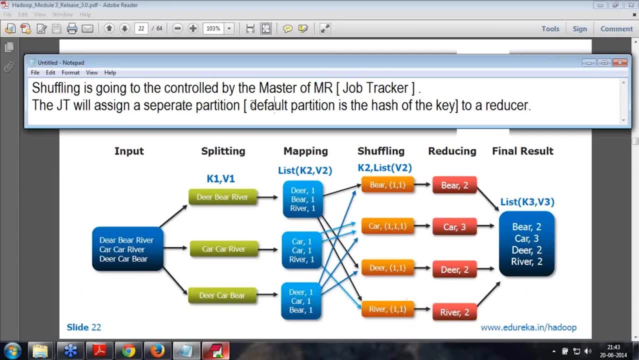 when the mappers finish the JobTracker will say that, okay, it will look at. if you don't say anything, it will look out for the default hash of the key and it will assign separate reducers to take care of the all the values for the key. friend, okay, so this is what. 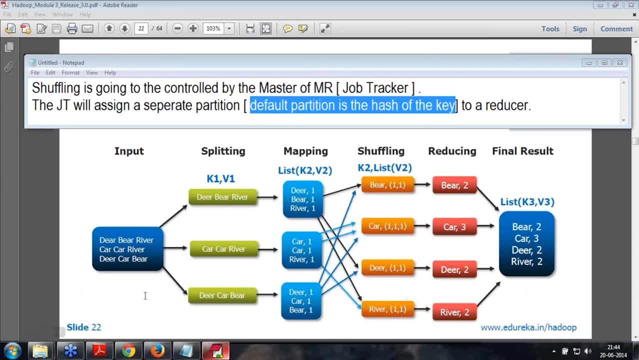 is going to happen. Hey, Shishobit was saying: default partition is the hash of the key. what is the hash? Hey, Shishobit, and Vasu hash is how it will calculate the ASCII value of any key. so hash. 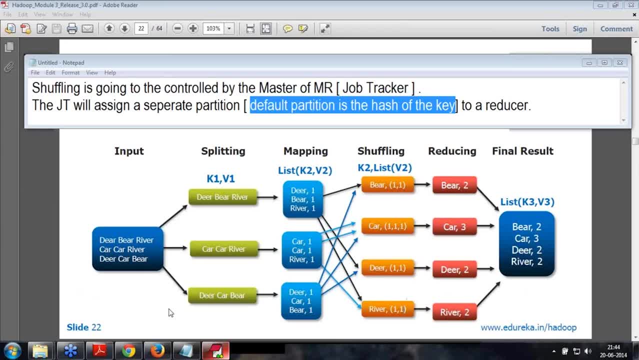 is a mathematical algorithm and all the similar values will always have the same hash. think of it like the ASCII value and the addition of the ASCII values. okay, so go down to Google and search for how to calculate the hash of the key. 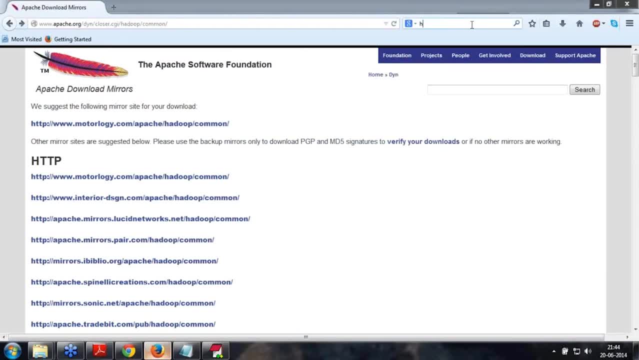 Okay, Shishobit was saying: default partition is the hash of the key. what is the hash? Hey, Shishobit and Vasu, hash is how it will calculate the hash of the key. that will give you an idea how to calculate hash of a key. okay, so it will show you a mathematical. 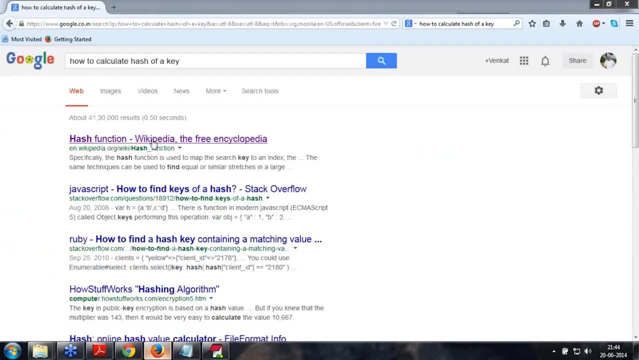 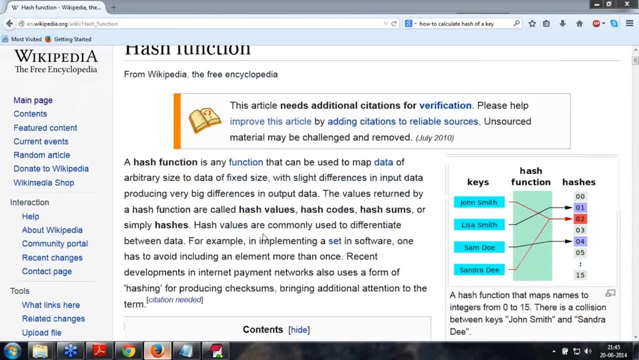 logic of how to calculate hash. there it is. so this is what is a hash function. okay, so you will see over here. the hash function is any function that can be used to map data of arbitrary sizes to data of fixed size. 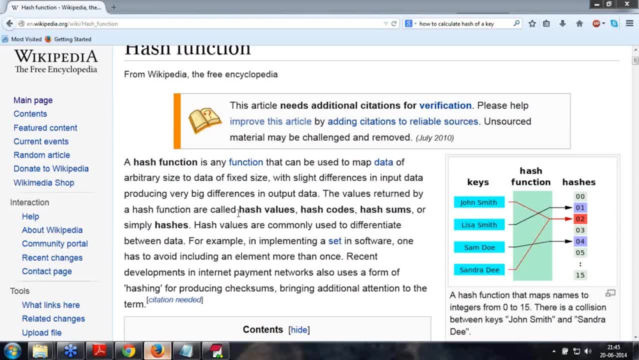 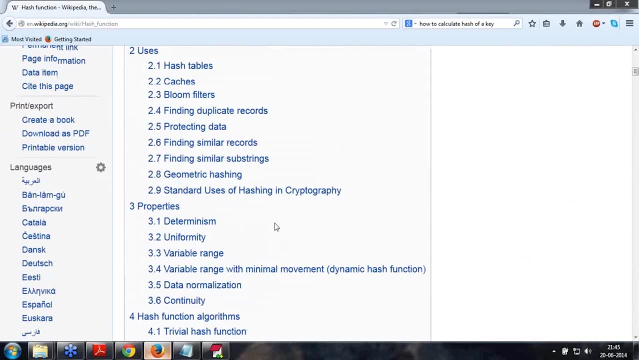 Okay, so the values returned by the hash functions are called as hash codes. in Java, there is something called as hash code, and you will see that both of your similar keys will always have the same hash. Okay, so there are various ways in which you can do that. since this is Java, it will look. 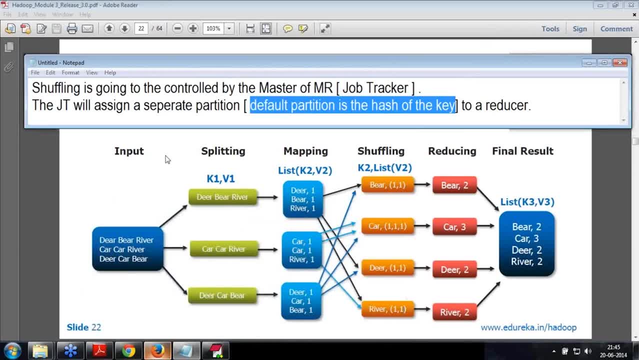 at the hash code, friends. Okay, make sense. So Sapnal was saying: reducer will act on the hash code. Okay, so what is the hash code? act on the list too. yeah, yes, let's wait, let's finish the uh shuffling phase and then we will. 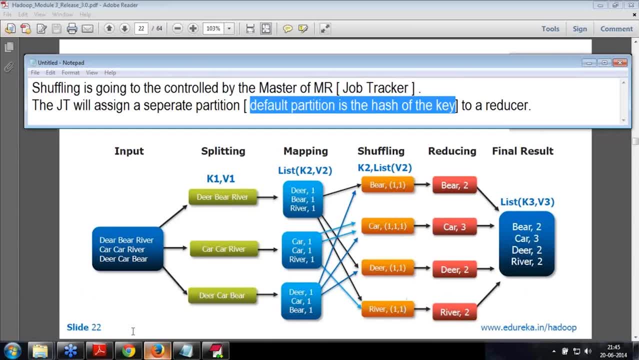 look at the reducing phase. funny was saying why beer is first in the order and not dear. okay, it depends upon how the hashing is done. okay, so typically when you do the hashing, it will always try to sort it. okay, when you do the shuffling, it is always called a shuffle and sort. it will try. 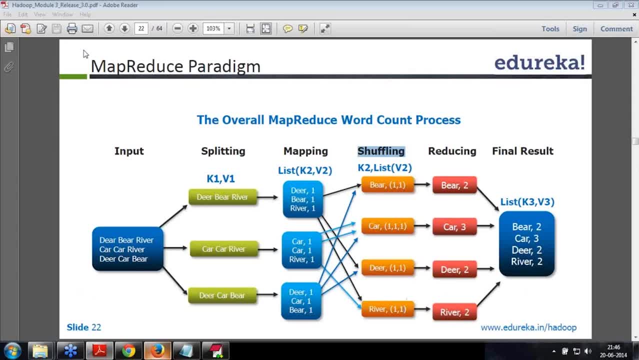 to sort it individually, okay, so good. so that is the reason we haven't gone to the word reducer until now. friend, a reducer is another component room where there is a map and a reduce. a mapper is going to be one guy who is going to do the mapping, okay, and the reducer, similarly, is another. 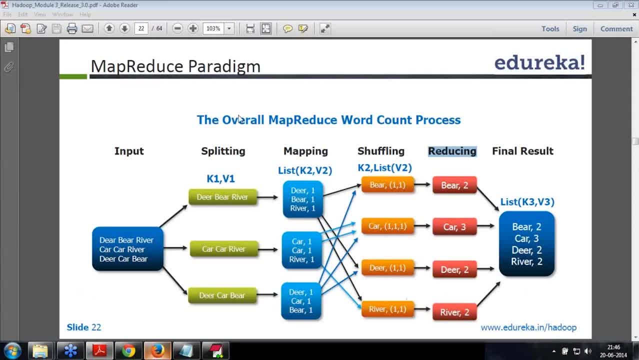 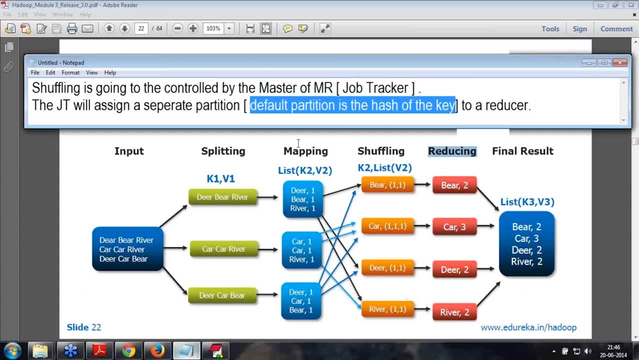 guy who is going to do the reducing. remember, yesterday we have seen the number of max map task and reduce task. right, Ravi? cool, so let me go back to my diagram. so this is what is the logic. so let me look at the questions window again. good, Ravi, so others. are you clear with what is the mapping phase? you write the. 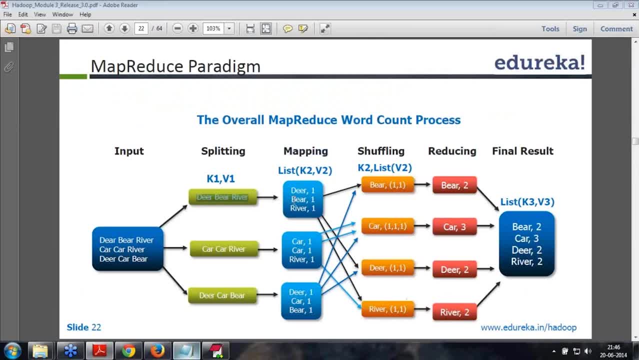 business logic of what you want to get from the record. you will get a list of keys and values. the shuffler, that is, the job tracker, will then look out because where is the shuffling process going to run? the shuffler will run the shuffling process and the shuffler will run the shuffling. 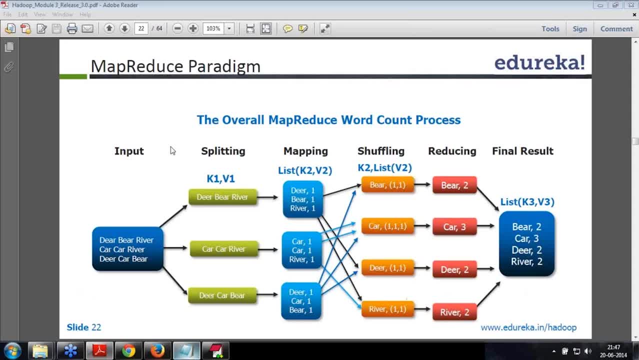 on all the map. that is executed on all the nodes. where was the mapper running? mapper was running individually. it was running parallely on all the nodes where the data was. as and when the data gets finished on any of the nodes, the shuffling will have to happen on all the nodes. so this is very 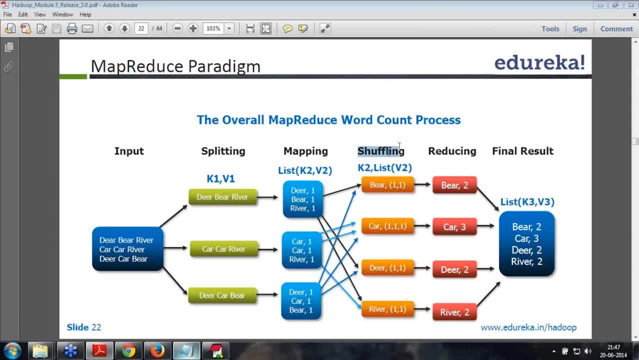 very, very important guys. so the shuffling process is going to go through all the nodes and once the data is finished, what will it guarantee is it will give you unique, sorted list of keys and all the values for the key will be given together. okay, so show bit, internally it will do different things. 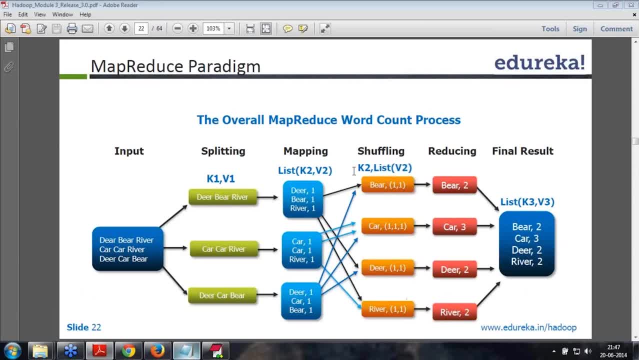 it will use some kind of collection. so it is going to use some kind of collection. so, whatever the guarantee of the, after the shuffler is finished all the keys- or the- I mean all the values of a similar key- are given to one another. after the shuffler is finished, all the keys are- I mean all the values of a similar key- are given to one. 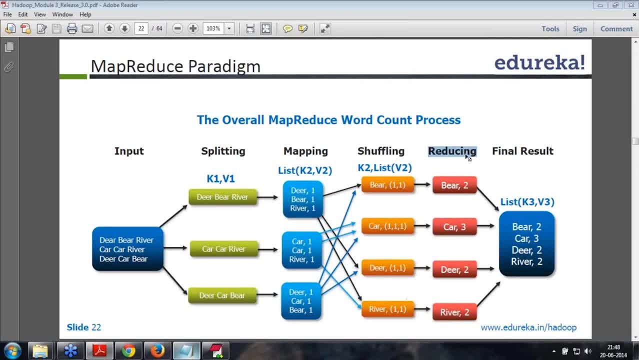 reducer, okay, and then the reducer will start working. so I just want to check if you are clear with the mapping and the shuffling phase, all of you. I would need communication right now. guys, if something is not clear, let's bring it up right now. so something was saying. so actually splitting: 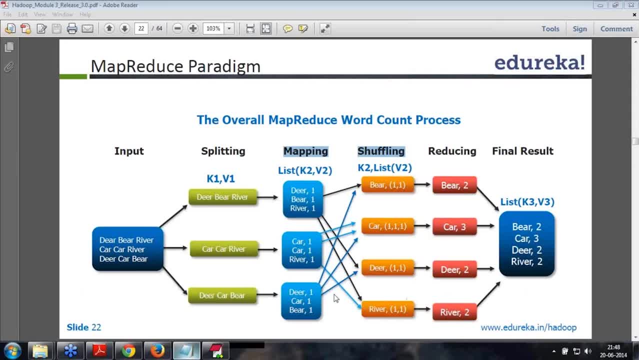 mapping, shuffling, all done physically on data nodes. exactly, the data nodes are the place where all of these things are going to be executed. folks, I hope it is clear for all of those who are very, very quiet today. okay then, my is not there for some reason today. 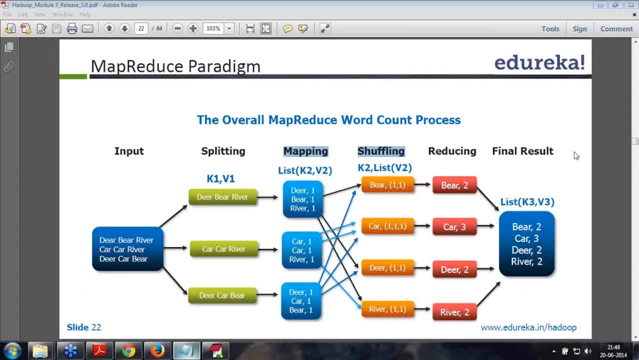 Sapna, you were there yesterday, friend, so I don't recollect, friend. so please, please, ensure that you are all clear on this. very good, Krishna. thank you, exactly, Srikanth. okay, Tanmay is not there. so they, okay, you guys are together. okay, so that's fine. so shuffling is done. 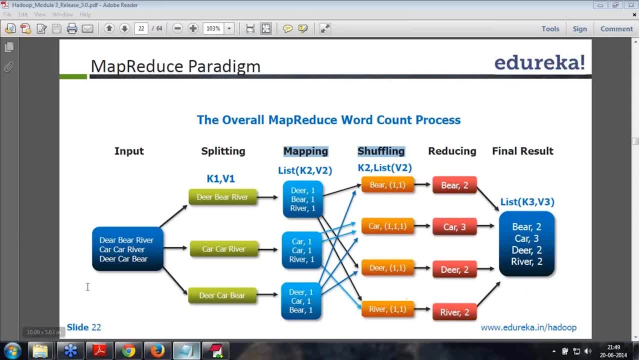 centrally. that's correct, so Swami said so. beer card dear has to be in an alphabetical order from top to down. that is what the shuffling phase will ensure. it will be sorting and shuffling. okay, so Amira can plus saying: can you write it down, the mapling and the shuffling phase on the? 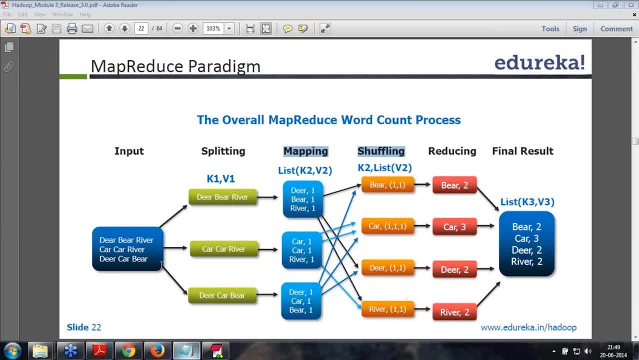 notepad. okay, I'll do that. yes, funny, shuffling is done across the nodes. only when it is done across the nodes, then you will get this because it key will be there on multiple nodes, right? so that's the way how it will work. proper is saying: do a node can accommodate many mappers and reducers at. 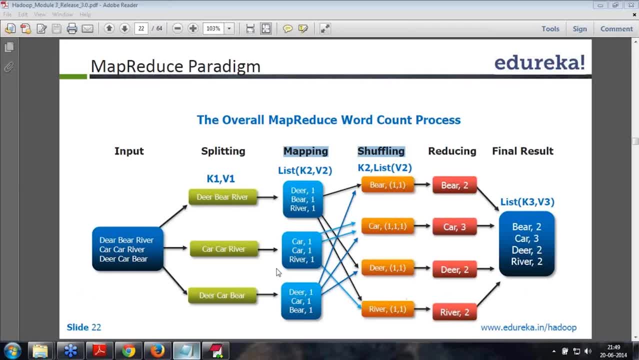 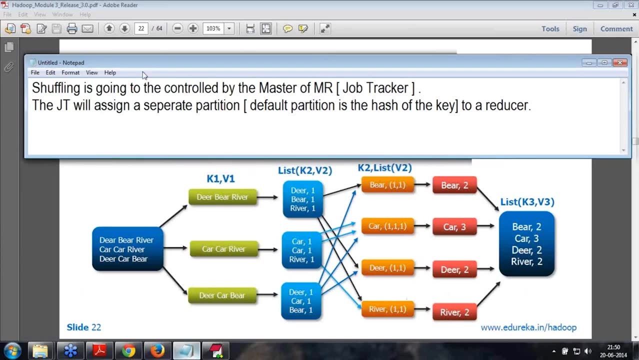 the at a point of time. yes, you can do that. remember yesterday we had max map task and reduce task. we had to write purple. we had it yesterday, right, good, good. so if you look at the reducer, so what is happening? there is no need of Nikon to write it down, it's over here. it will look at the key of every it look. 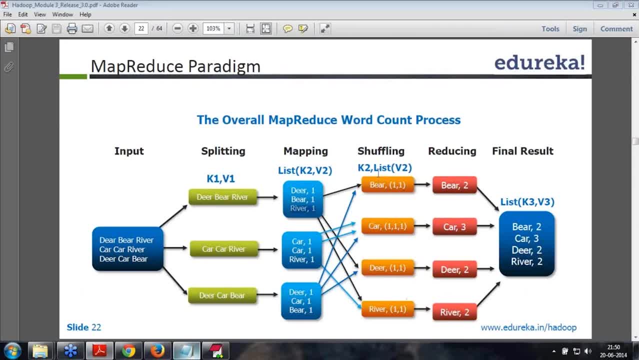 at the output of every mapper and then sort it and then start assigning it to different reducers. so once the shuffling is done across all the multiple machines, okay, you will get a key and a list of values of Nikon. that it clear on this. what did you want me to write it on the notepad, friend? I was not very clear on. 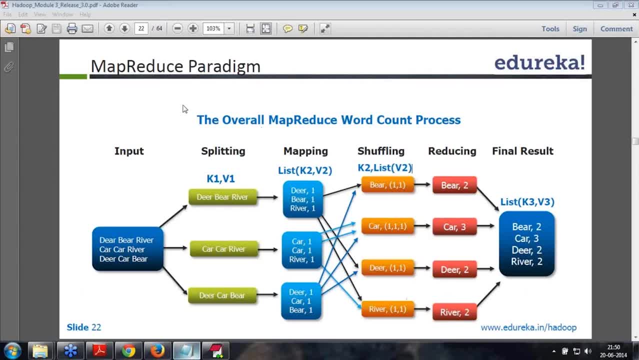 what you want me to do, friend, because the diagram is very clear. where is the shuffling done? what memory does it use? the shuffling is controlled by the job tracker, but is actually done by the task trackers. okay, so the memory of the task tracker is used over here. 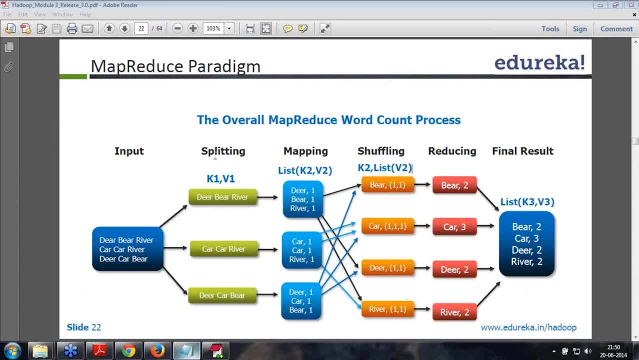 funny, sure, sure of Nikon. okay, so, depending upon the max map, we are along the same data set will be executing different logic. mapping and shuffling can be done. hey, first mapping needs to be finished on a record, then the job tracker will have the date unknown to the shuffling processing. that means 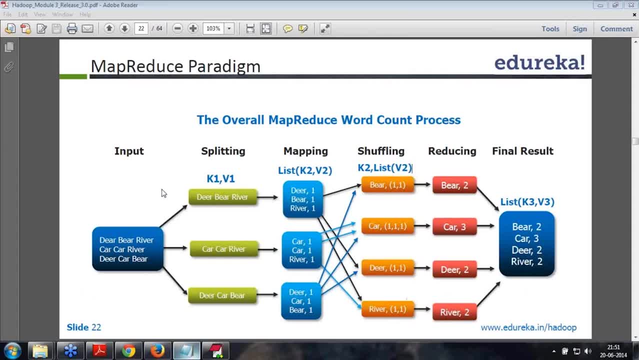 see there is cross, cross movement of key values, you're right. so all those movement of key valises controlled by the job tracker, by the master right, good help to karate team. Funny was saying, when there are individual job trackers and task trackers for each node. 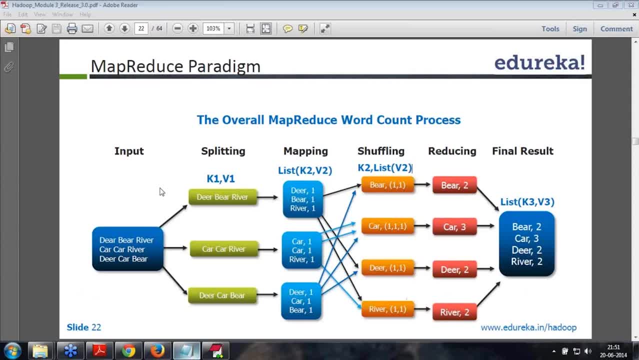 then which job tracker, task tracker memory is used? Hey, where will the mapping happen? funny, On the nodes where our data is right. So let's assume I have got 10 node cluster. I have got 100 MB file. 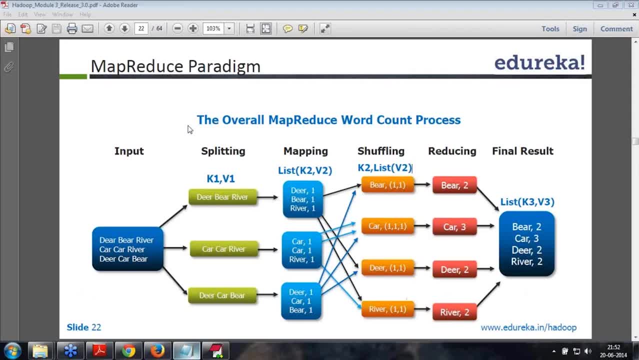 So how many nodes will have the data? Two nodes. So where will the mapper run? Only on the nodes where the data is right. funny, But where can the red users be running? Let me get the answer. I have got 10 nodes. 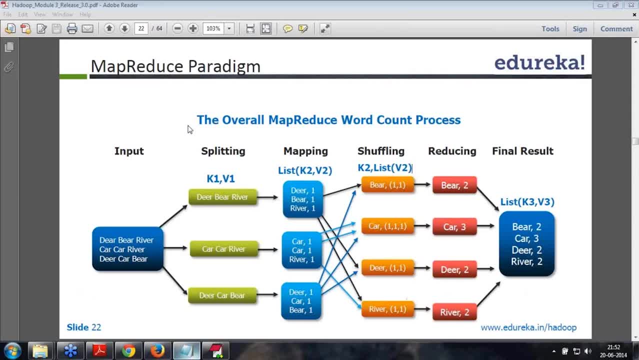 64 and 36 is on two nodes, So mappers will run only on two nodes. Where can the red users be executed? On two nodes or on 10 nodes? Why two nodes, guys? Why do you think it's going to be only on two nodes? 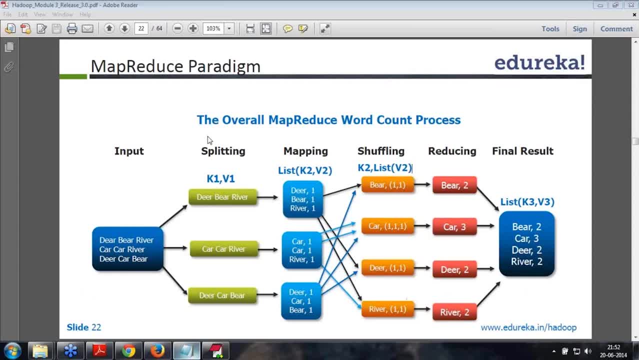 It will be 10 nodes. That's right, Srikanth, It will be 10.. Why 10?? Because you see, over here there are three mappers, but how many red users are there? right, There are four red users, right. 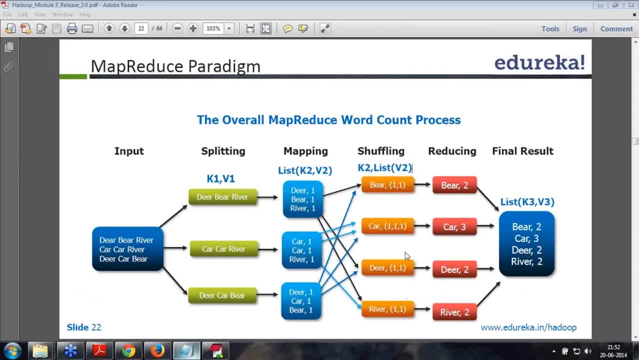 So, don't you see? there are four separate red users. So each of the red users can be done by separate nodes, right? So it's the shuffler which will decide all the resource management. So who is going to do the shuffling work? 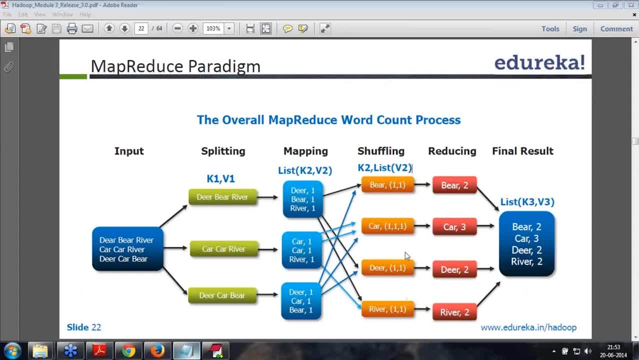 Depending upon which reducer is going to do the shuffling work, on which node, depending upon the resource utilization at that point of time. Mapping is always done on the node where the data is: data locality. right, But now there are three mappers. okay. 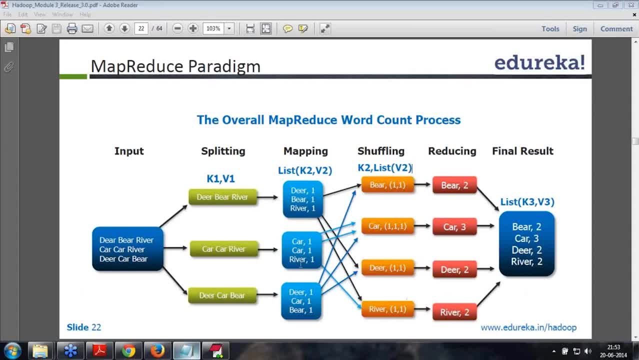 But then there are four red users, right, You can see it on the same screen. So that's why reduce can be done on any node in the cluster. So people typically think, hey, there will be a network choke-up because of the data movement. 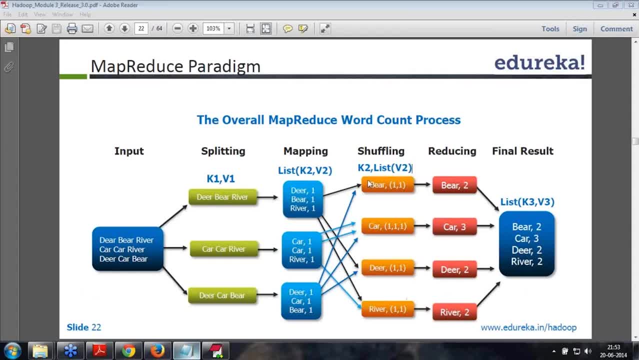 No, It's all done Not at the same time. So when one mapper finishes, imagine I'm a courier company and I have got 10 people who are going to get me couriers And I typically give the courier to four states: Delhi, Mumbai, Calcutta and Chennai. okay, 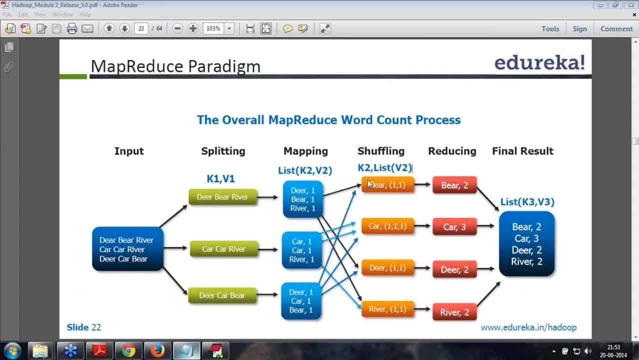 So do I have to wait for all the 10 courier guys to come and then do the arrangement? No, Whenever one courier guy comes, I can do the arrangement right. So the shuffling starts immediately when one mapper output is finished. okay, 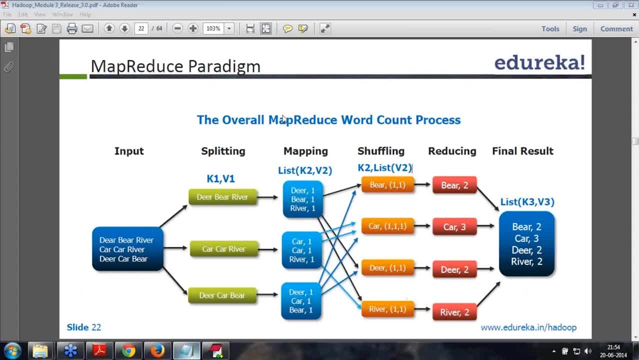 Okay, But then the final summation of all the envelopes for Mumbai, Delhi, Calcutta and Chennai will be done only when all the 10 guys have come in right. So the shuffling work starts when the actual one mapper have finished. friends, 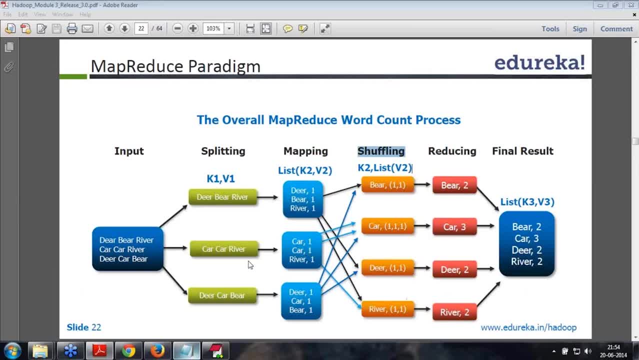 Cool, Cool on this. guys Understood this. What does reducing and shuffling So funny said? So it means shuffling and reducing can be done on any, Any node. no need to happen only on the nodes where the data is residing. 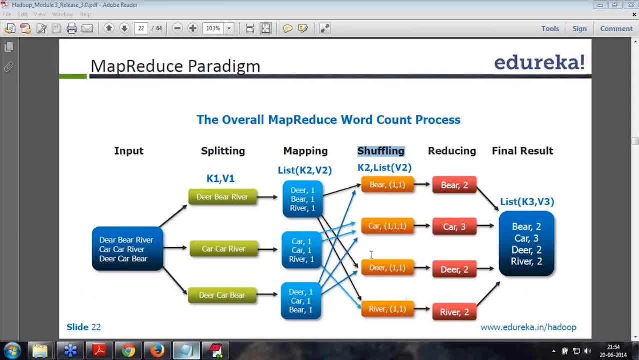 Exactly funny, That is exactly correct. Okay, Very good. So Apnil said I mean same record data set can be processed at the same time with two different logic, That is splitting and mapping. Hey, splitting has mapping Before mapping. you should have splitting, right. 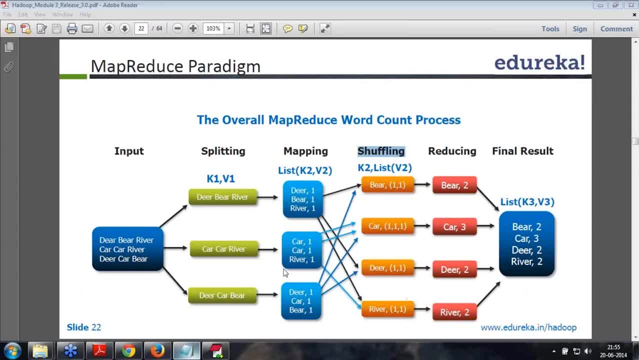 So, because there is no lock needed over here, because it's right One, You can have multiple analysis working on the same data set. You can think in that way. But before mapping I need shuffling splitting to be done, right. 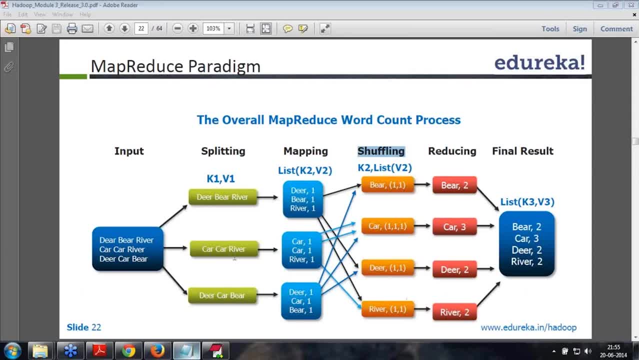 Good. So Wasu was saying number of mapper machines is equal to number of reducer machines. No, No, No, No, Wasu, Because number of mapper is dependent upon the size of the data. So if your size of the data is, let's say, 100 MB, 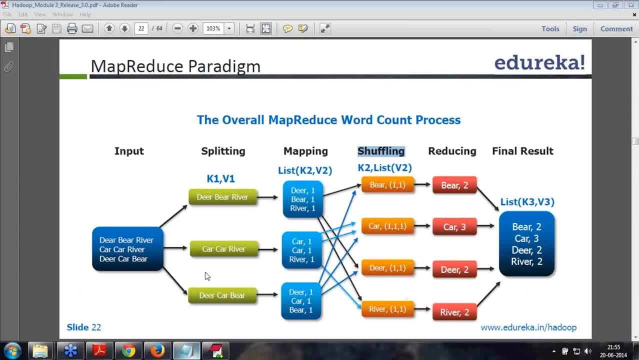 you will have it on two mappers will be running on two machines. The number of reducers will be dependent on the number of unique hash of the keys right. Look at the screen: You have got four reducers, whereas you have got three mappers right. 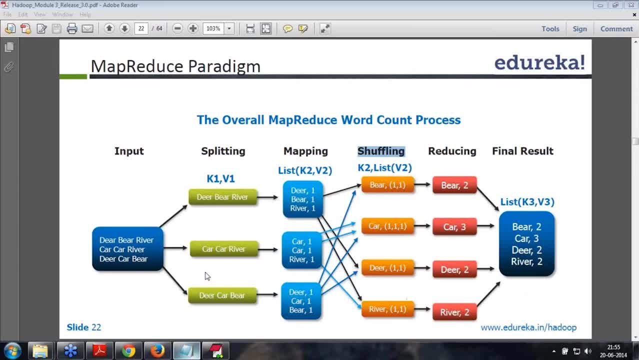 Wasu Dave clear on that Exactly: Reducers would be dependent upon the data content. That's right. How many reducers needs to work on it is going to be dependent upon the data content. Very true, Very true, Make sense. 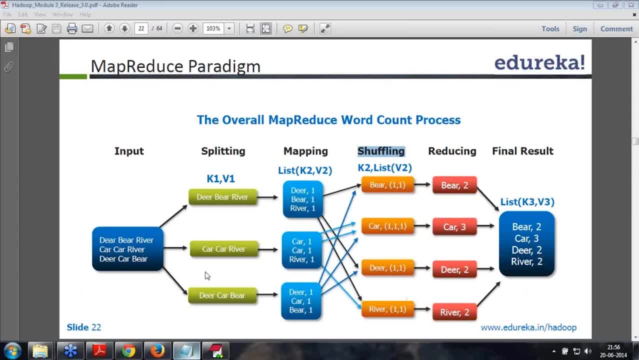 Good, Good. So Prappal was saying I expect that there will be a lot of data exchange and comparisons at the time of shuffling for a big file. Why do you think there will be a lot of data exchange? Yes, there will be data exchange, but is all the data exchange going to happen at the same time? 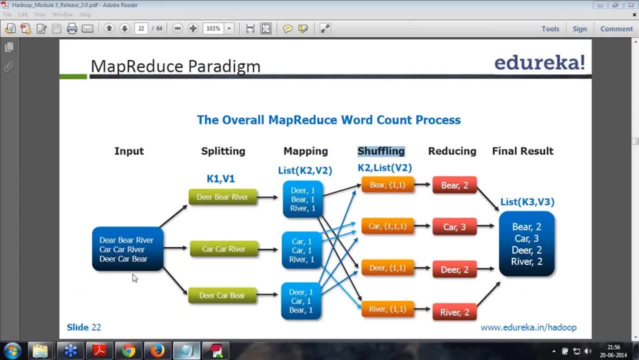 No, Right, Because if you have got one million lines, okay, will all the one million lines be processed parallelly? No, It will be processed based on the number of data. It will be processed based on the number of mapper slots. what am I having? 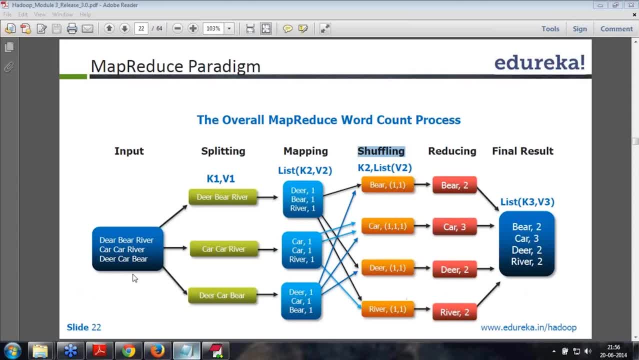 Imagine you are a BPO company and you have got ten employees. How many calls can the ten employees take at one point of time? Prappal, I have got ten employees. Okay, How many calls can it be taken at one point of time? 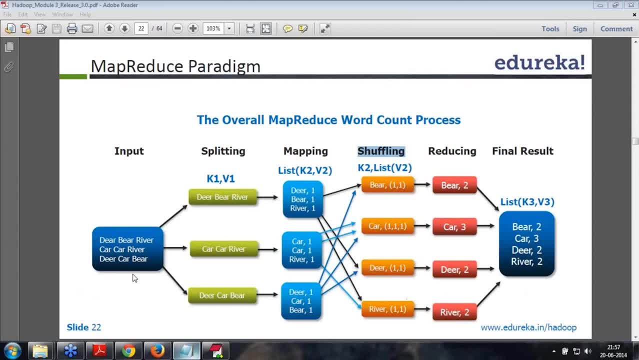 Ten. But does that mean in a day I can take only ten calls? No, right, Right Navdeep, Right Sapna, I can take multiple calls. right, Getting an idea of it? Yes, So the moment one of the calls finishes, he can pick up another call. 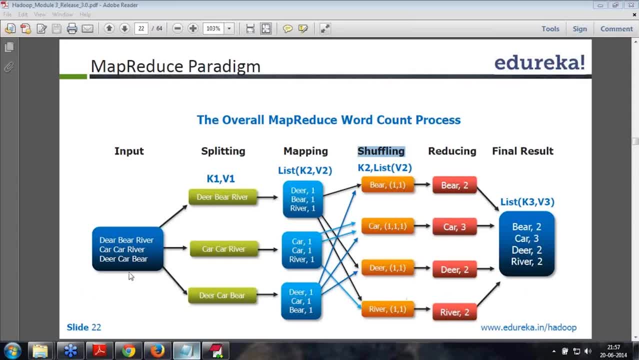 These are all small records which can be analyzed real, real quick. Good. So Ravi was saying: if you want to split based on the letter instead of the word, we will have more reducers. Is that correct, Exactly, But you will have maximum 26 reducers depending upon the number of unique words. 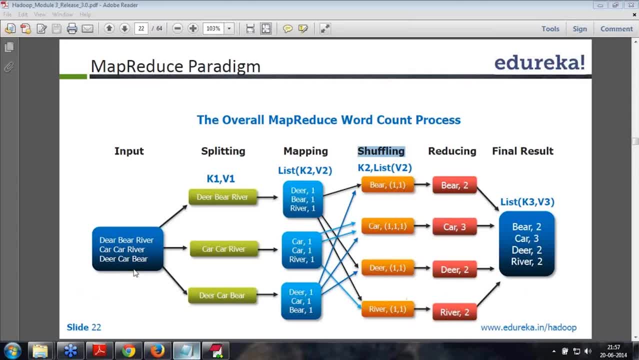 You won't have more than that right. So imagine, if you want to do a word, let the word count of how many words are used in the in a Shakespeare's novel. okay, maximum number of reducers will only be 26,. number of unique words: right, Ravi? yes. 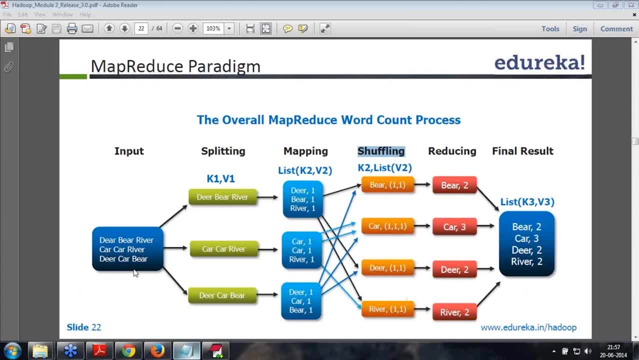 Make sense. Good, Hey guys. why am I giving you these examples is because I want it to be clear, friend. Okay, Don't take it in a wrong way. I am giving you these multiple examples so that I want you to be clear. 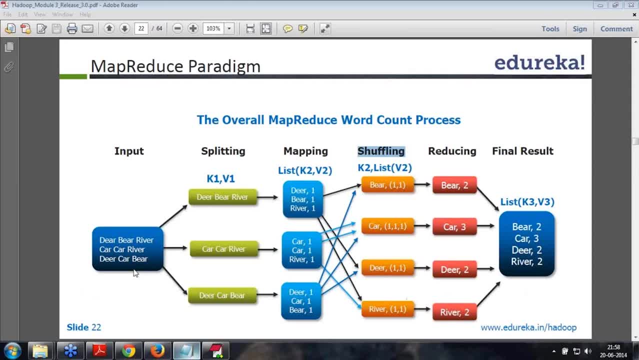 There should be no doubt that is going to be there in your mind. Nobody should be able to confuse you after taking my class saying that, okay, what is my problem? Nobody is probably going to actually produce. they should be able to shake you. 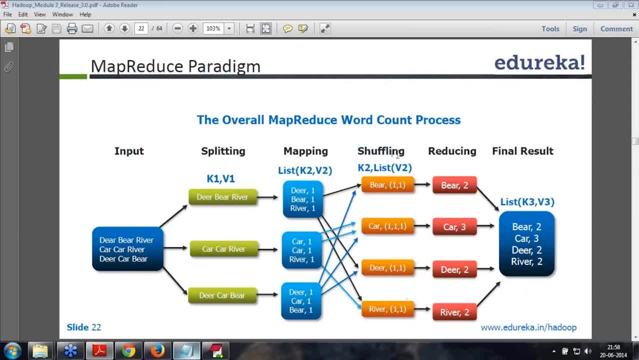 Good, So let's carry on, friends. So now I am going to shuffle. okay, You know the number of unique keys. that is there, right? Hey, before I go ahead, Abhana was saying that right now we know there are three records. 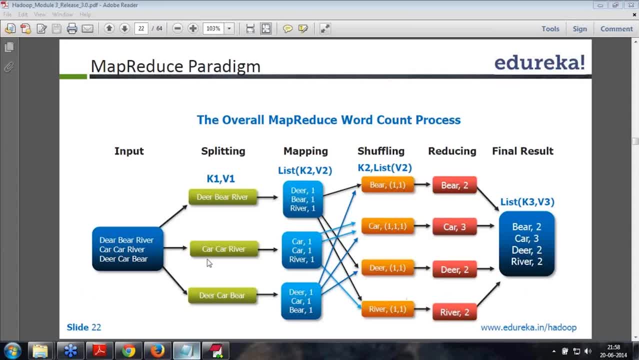 One card has four words and the other has got three. How many maps will be used? three or four? Okay, Abhana. maps that will be used is the number of records. okay, so if you have got three records and one records, okay. so the number of maps runs will be dependent. 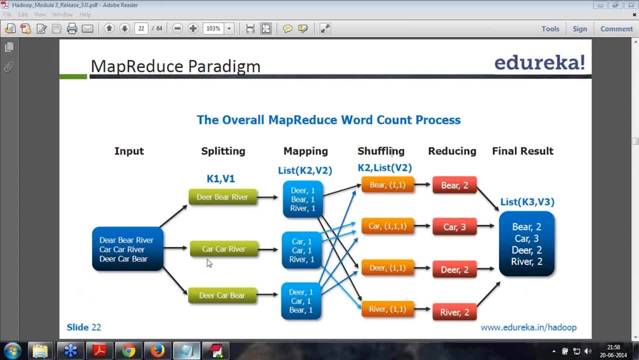 upon the number of records. it has got nothing to do with words in the mapper, is what you are converting a record to a word. right, make sense, Abhikant, good, good, so if you have got three records, you'll have three maps. you write the logic of. 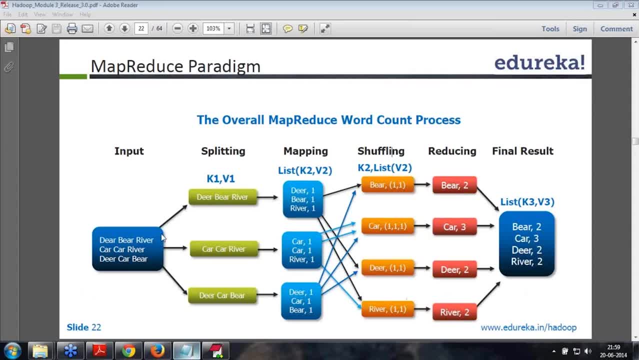 it, then the shuffler will ensure that all the unique, all the values of the unique key will go down to one reducer and then it will do the reducing part of it. simple, fantastic. so after the shuffler, you will get something called as your key and a list of values, okay, and then you will have the reducer and 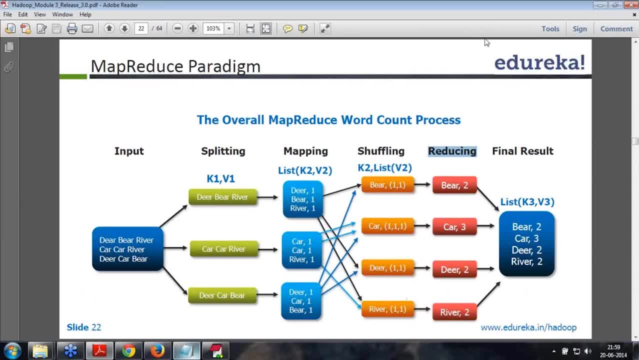 then you write a reducing logic. in this example, you want to do a sum. in the transaction example, you want to do a sum. in the temperature example, you want to do a max. so the reducing always does some kind of aggregation and then the final data is what is stored in your 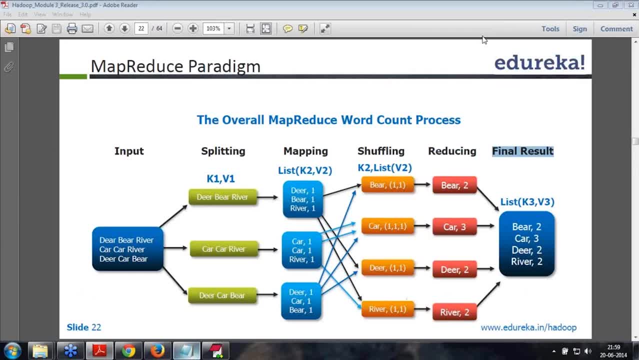 final result. so this is what does the overall map reduce word count process. okay, so hope it is very clear for you as to how we can do an end-to-end process for the map reduce. so these are the six columns. input is the data one block splitting decides how to identify a record in the mapper. you write the. 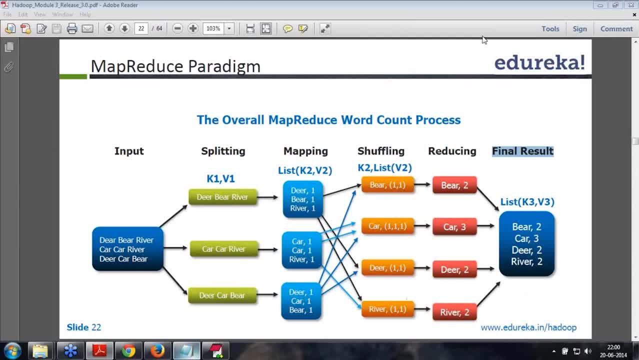 business logic of what do you want to pick up from the record? shuffling ensures that all the values for a similar key across multiple data nodes, wherever the data is written, is all given to one reducer. so the default partitioning is based on the key or, sorry, on the hash of the key. okay, supposing if you want to say that all. 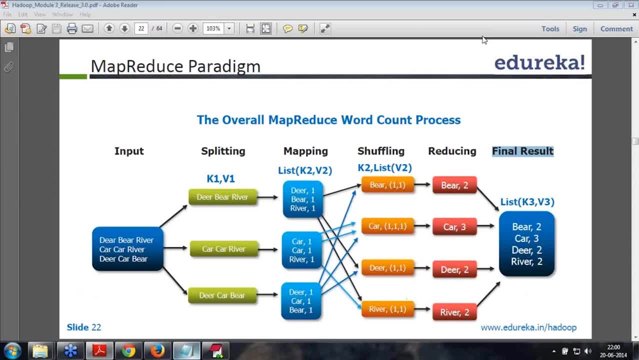 alphabets, all keys starting with ABC should be one and greater than C should be another. okay, so you will have beer and car going to one, and then, in this example, deer and Rover that is greater than BABC going down to the second. so you decide what is your partitioning logic. depending upon that, it will go. 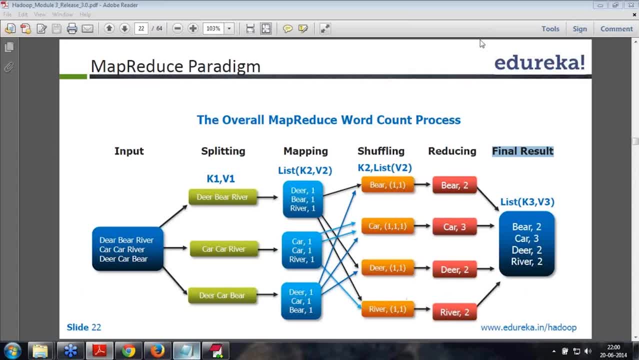 down to the reducer. the reducer will do some aggregation and the final output is what is going to be stored in HDFS. exactly. so if you say ABC should be in one and greater than C should be in another, there will be two reducers. exactly, that's right. that's right. 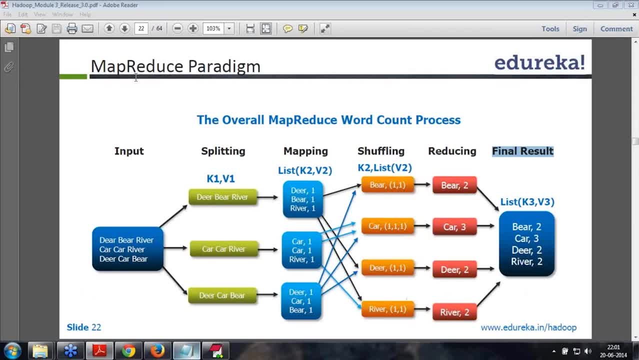 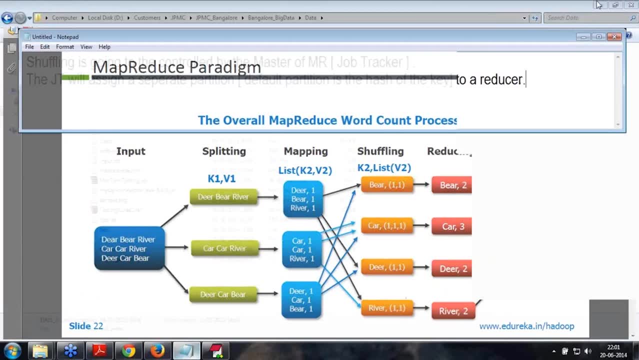 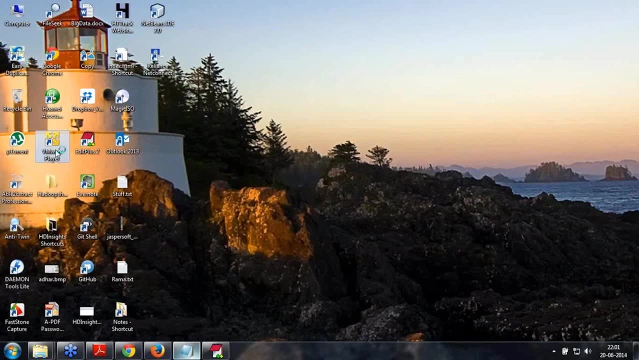 stop now. okay, so fantastic guys, a couple of slides and then I will stop, and then I will give you a demo so that at least you can see how to start with things. so what I need to do right now is I need to real quickly start with my VM player, because I need to give you a complete demo of this. 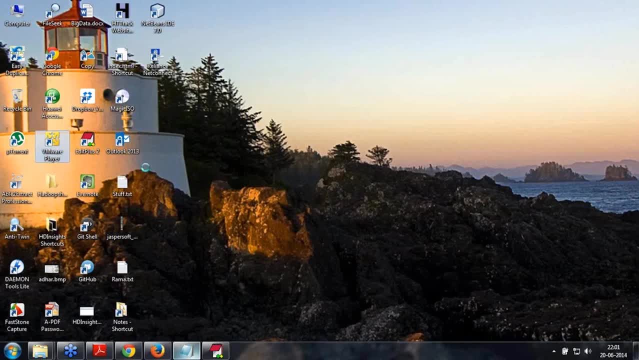 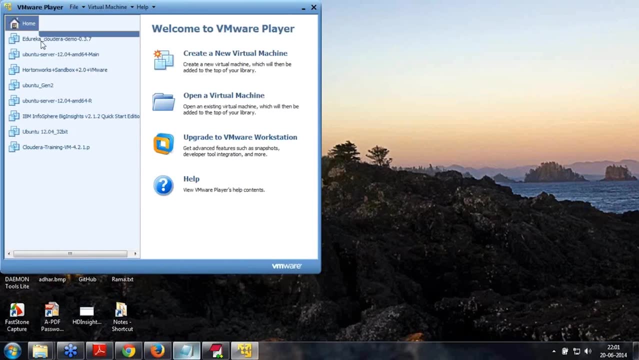 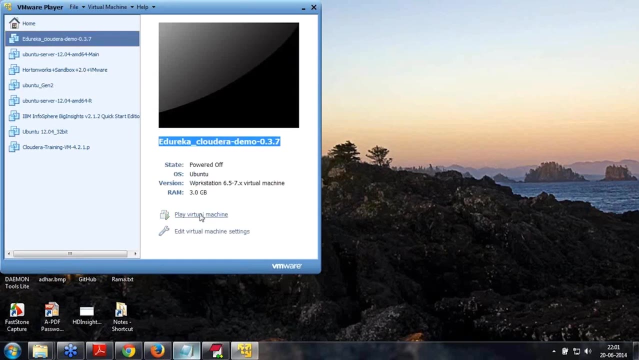 before. of course there is a video recording, okay, so you can look at that map, reduce program video recording also, so that will also give you a very good idea. but then I thought that I will show you the complete runoff it so that you will get a hang of it. so let me go ahead and say: play the VM while the VM is. 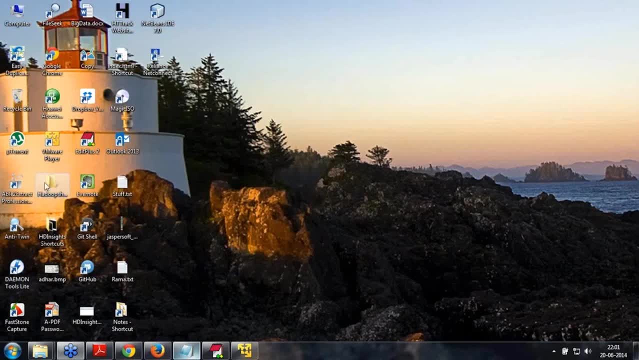 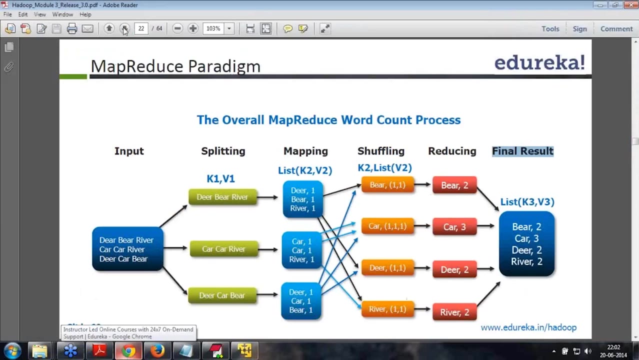 going to be played. let me minimize it. let me start with my Eclipse and let the Eclipse come up. so in the meantime, I'm going to go down to my next slide. so what are we doing over here in? the next slide is going to be: we are going to talk about the anatomy of the map. reduce what we 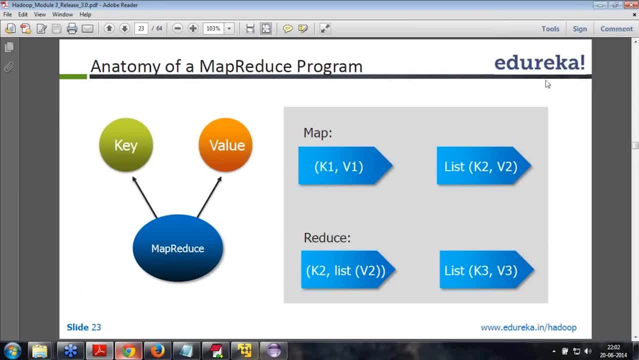 have just discussed right now. so everything is going to be a key value. the input to the mapper is going to be a key and a value. what is going to be the key? the input to the mapper. here, guys, what will be the key as input to the mapper? 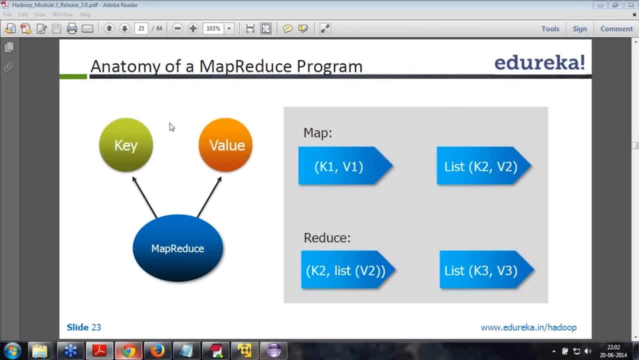 what will be k1 here, guys? what's the answer? what will be k1? very good, cursor position or offset point. the value will be the whole record. very good, Ravi, very good Krishna, okay, good, good. so then the mapper will ensure that you will do the business logic and reduce the value of the map, reduce the value of the. 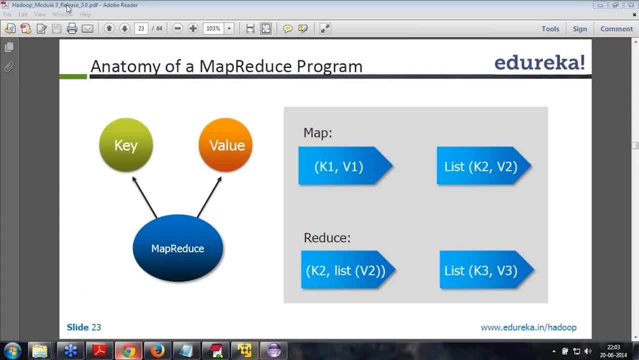 return a list of keys and values. very good, Shishobet right Srikant right Soumya- sorry, right Soumya. and then the shuffler will ensure that those list of keys and values are shuffled, so that you will get a key and a list of values and then in the reduce you write the business.